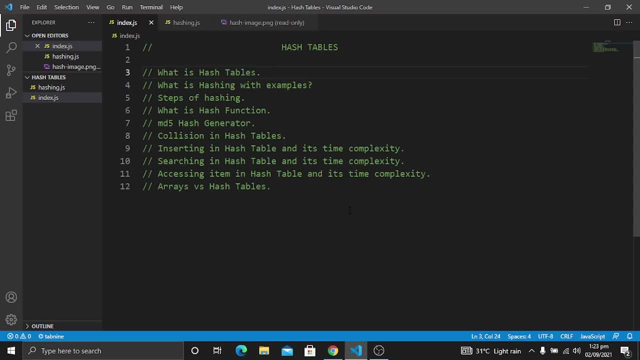 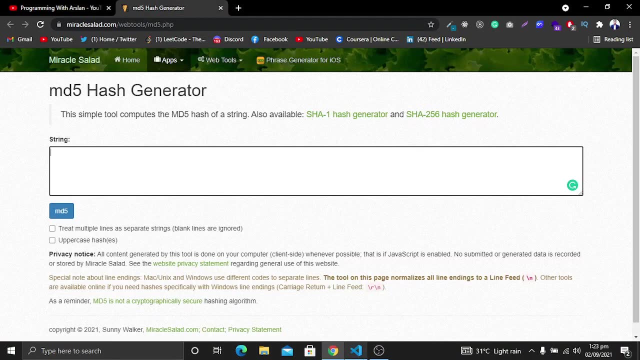 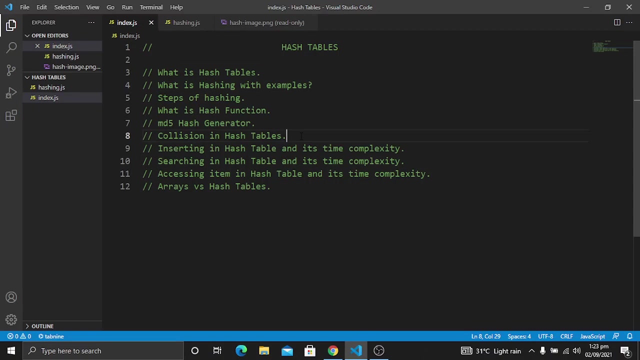 So what does hash function do? And then we will learn about the MD5 hash generator. So in this website we will learn what is this? Now, in the next step, we will learn what is collision in hash tables And what we can say is: how can we solve this collision issue. In the next step, we will learn how can we insert in hash tables. 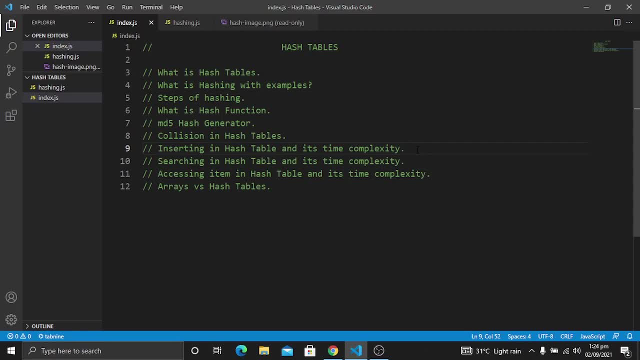 Then we will learn how can we calculate its time complexity or what is its time complexity. Then we will learn searching in hash table and its time complexity. So how can you search in the hash tables? Then, in the next step, we will learn accessing items in the hash table and their time complexities. And in the last step, what we will learn is the difference between the arrays and the hash tables. 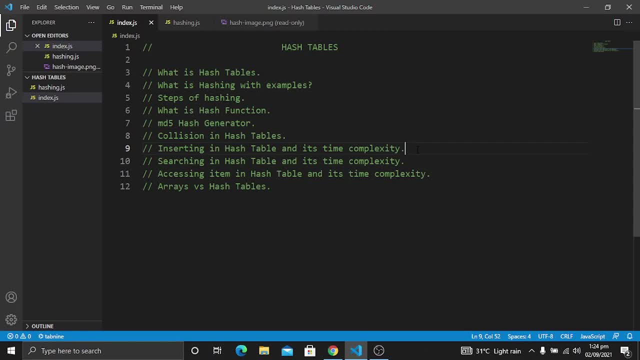 So the first step is: what is, or we can say what are hash tables? Data structure. So in hash tables key is passed to the hash function, Then it will generate address in memory where key value are stored. Or we can say key value pairs are stored. So basically, hash tables are just JavaScript objects, or we can say objects in JavaScript dictionaries in Python, hashes in Ruby, And there are different names for different languages. 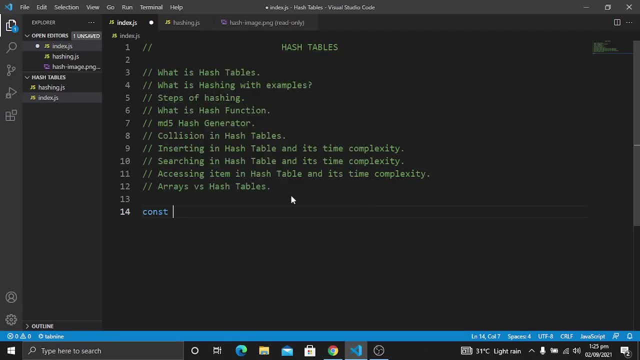 Which is first of all. I will give you simple example. For example, I will create an object here which will say, for example, name is going to be the Arslan, Then we can say: work is going to be software engineer, Then it is understand that this object is your job and then it will direct you to here And things happened to these objects here. so what not to say? and we can just use this object in memory. 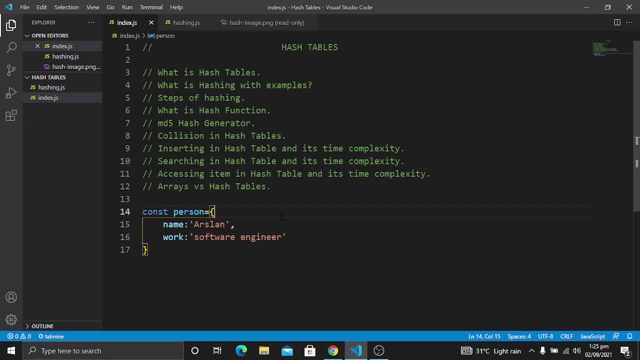 So here is the 2nd part of this tutorial to understand how can you search in the hash table and its time complexity. Then we will learn types of keys for which the parameters are different. Here: umpire not onlypaln is using connect object. 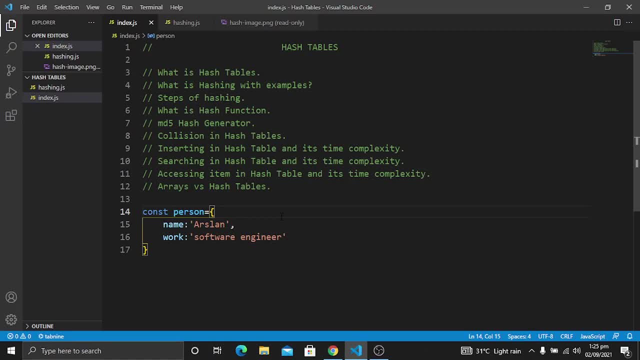 Then it uses every 2 hand sign. Let us write it as root key, and now we know the meaning of all this: deletion: accessing. so first of all, you have understood that these are dictionaries in Python or objects in JavaScript. what is their role? so they, they store data in the form of key value pairs. in the previous lecture, we have 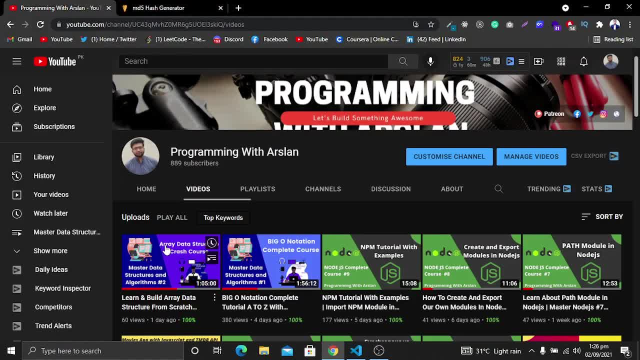 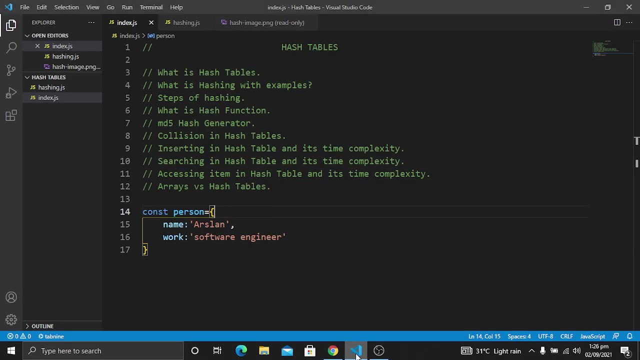 learned about the array data structure, so if you haven't watched this tutorial, I will recommend you to first of all watch this tutorial and the bigger notation tutorial. now, in array data structure you have seen the data is stored in the form of just the value, pairs and indexes. so the indexes are 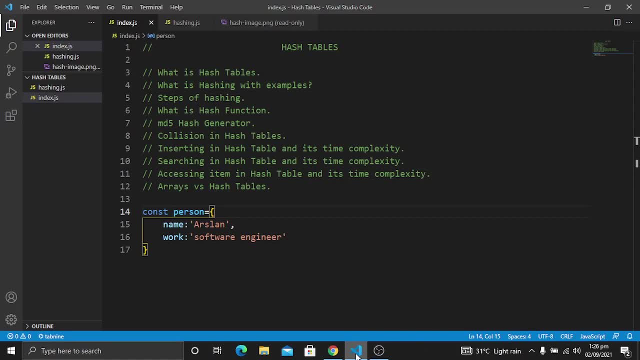 always in order. for example, 0, 1, 2, 3, they are in order and the values are stored in these indexes in the memory, whereas the hash functions are not in order. or you can see like this: these hash tables are stored in the memory as a key value pairs, not just the 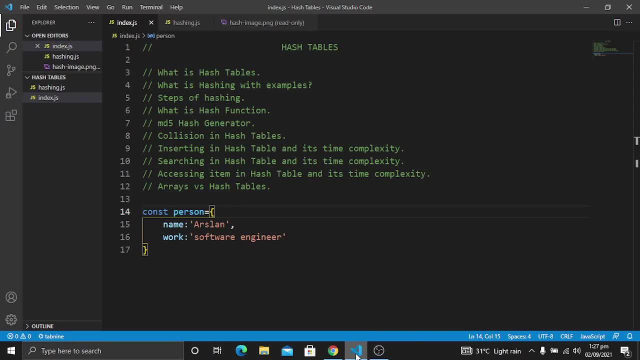 value. they are stored in the key value pairs. so, first of all, the keys have been passed to the hash functions. they generate the memory location and, and in these memory locations these key value pairs has been stored. we will learn about the whole process here. so, first of all, let's learn about the hashing in these hash. 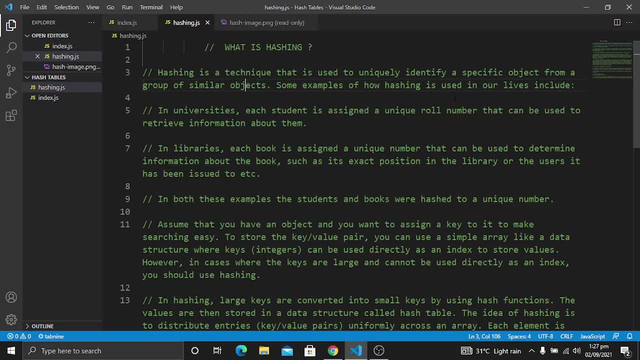 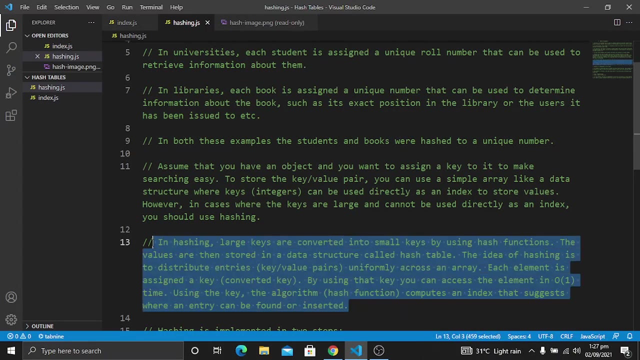 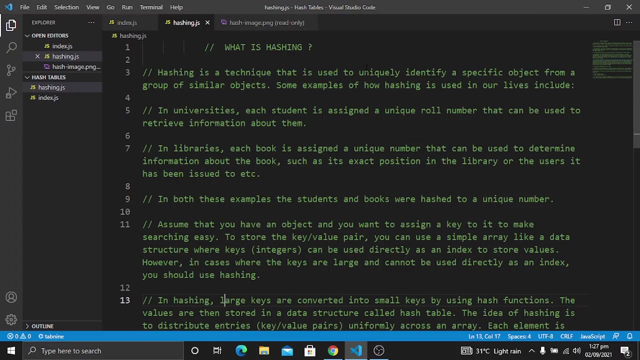 tables. so what is hashing basically? so here I have written the definition of the hashing or the, with the help of some examples, so these are from daily life examples. then here is a complete information about the hashing, what the whole process looks like. so let's start. first of all, what is hashing? so hashing is a technique that is used to uniquely. 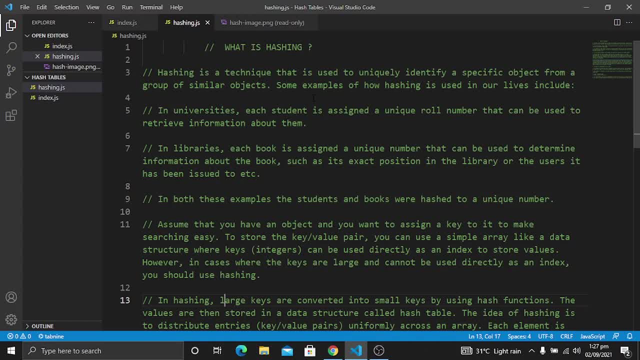 identify a specific object from a group of similar objects. some examples of how hashing is used in our lives include: in universities, each student is assigned a unique roll number that can be used to retrieve information about them. so, as you see, in universities, every student- or we can say in a 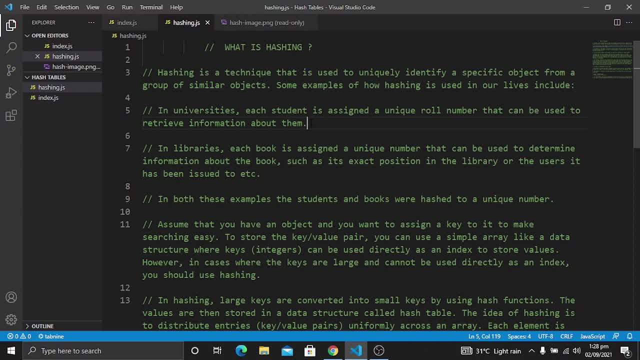 classroom every student has a different roll number and the information is associated with that roll number is about that student. so you can use this example so you can clearly understood the idea behind the hashing, that every individual element or student has a different ID, or you can say different. 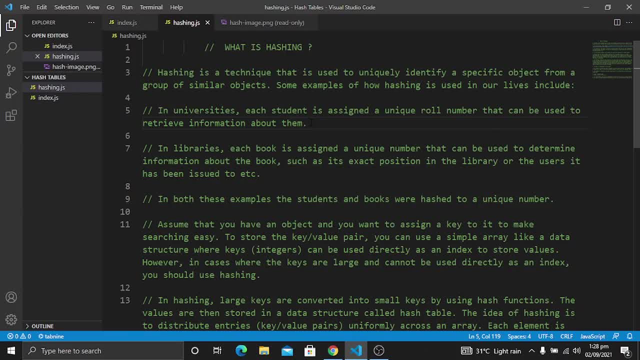 roll number. so in in those IDs are on this roll number, just that in the information of that user will be stored, not the all of the student, just the information of that student will be stored with this specific ID or with this specific roll number. in libraries each book is assigned a unique number. 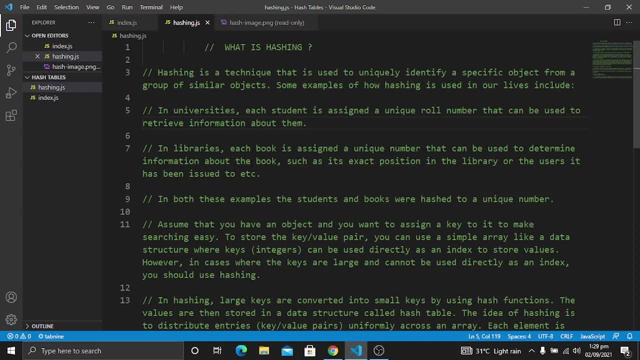 that can be used to determine information about the book, such as its exact position in the library or the users it has been issued to, etc. so, similarly, in the libraries you will see there will be specific memory location for specific books. so when you want to find the book next time you will know the location. 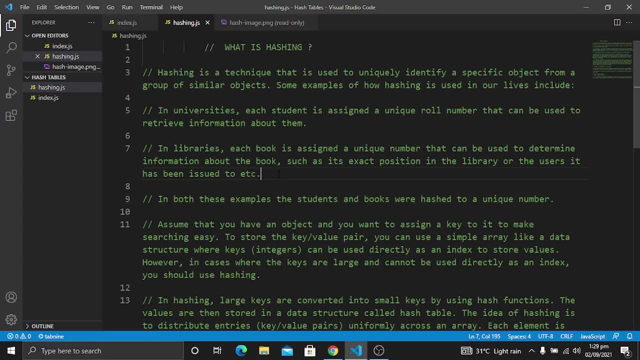 of that book. so you will move exact to that location and you will pull out the book and read the information in it and then you will store it afterward here. so this is the idea that every book in this library will have some uniqueness in it, so it will be easy for you to find that book or find the information. 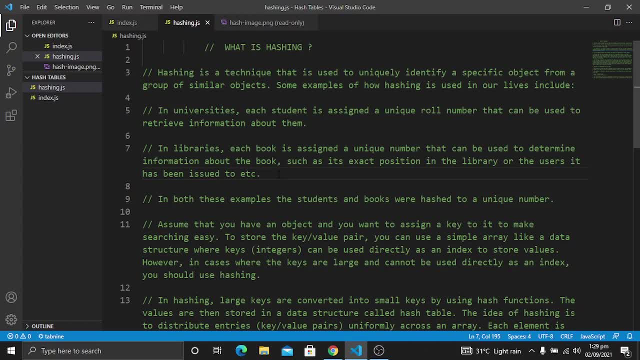 about that book. this uniqueness could be the name of the authors, or we can say the indexes, or we can say the some memory location, or we can say some memory positions with specific IDs. so this can be anything, this uniqueness. so in both these examples, the students and books, or we can say the student. 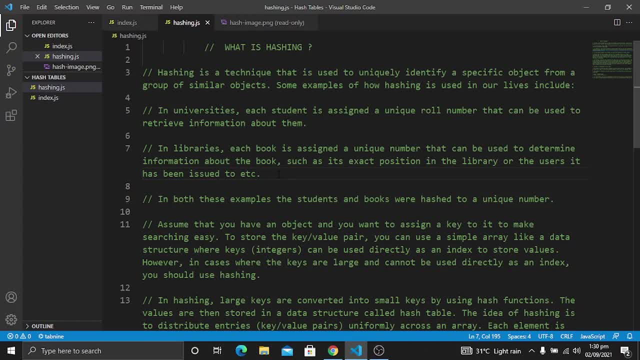 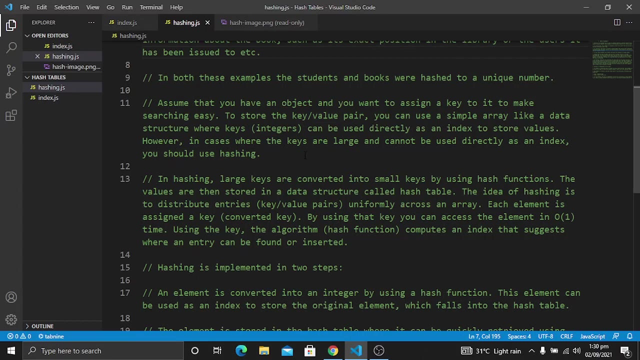 books were hashed to a unique number. so you will see the uniqueness is common here in this library, in both of these examples. now let's move towards the next paragraph. so it says: assume that you have an object and you want to assign a key to it to make searching easy, to store the key value pair you can use. 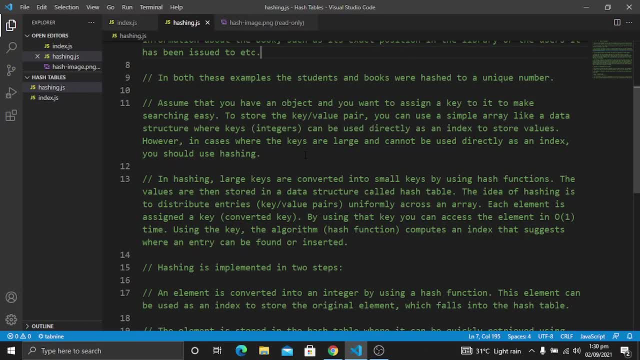 a simple array like data structure, where keys can be used directly as an index to store values. however, in cases where the keys are large and cannot be used directly as an index, you should use hashing. so what we can say in these hash tables? or we can say: 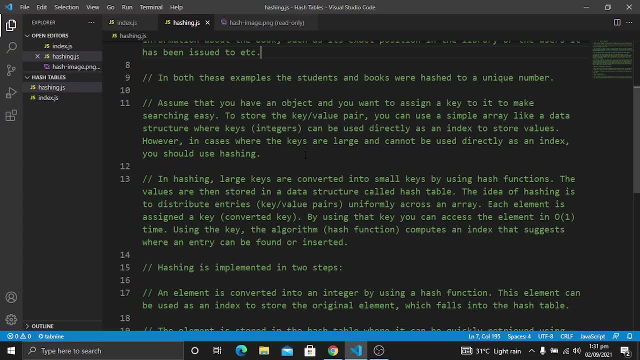 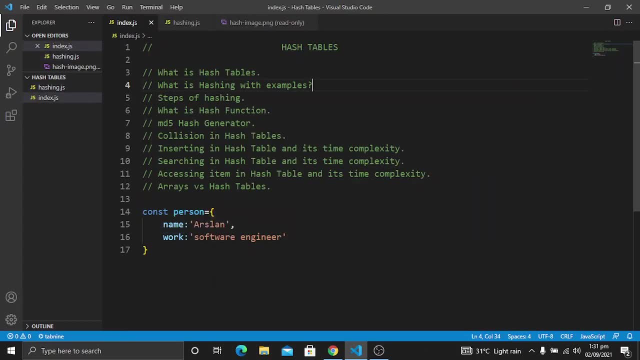 objects or dictionaries. what we'll do is, if you want to search something in the hash table, we can search with the help of keys. so, for example, the example that i have written here. so if i want to search about the information here, for example, you want to. 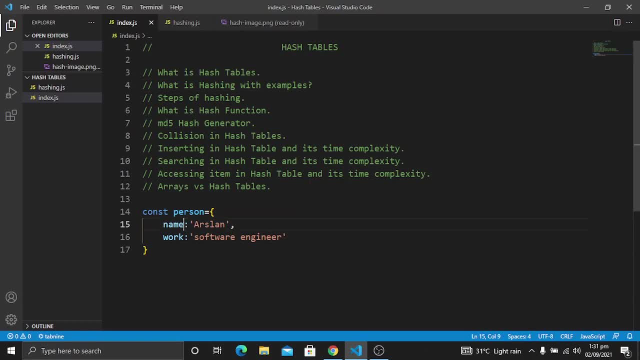 check the name. what i will do is i will use this name property, which will be, i can say, person dot name, to access this information. so these key values are. these keys are important here. so, for example, let's i will show you example, so i will consolelog here and 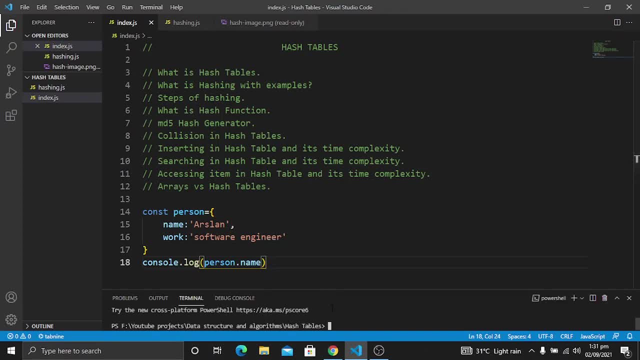 then i will use personname, then i will open the terminal. so clear the terminal. run the code, oops, indexjs. and i will see i'm getting an error here. let's see. so let's run the code again: node, indexjs. now you will see i'm getting the. 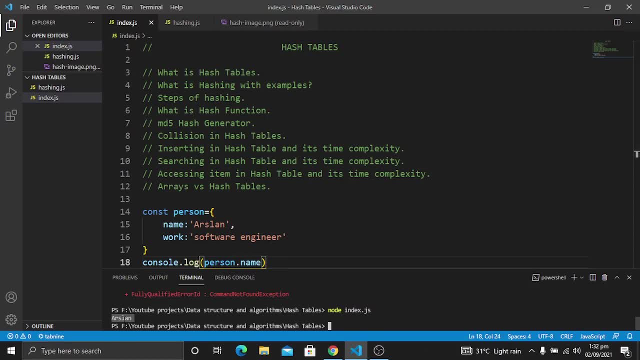 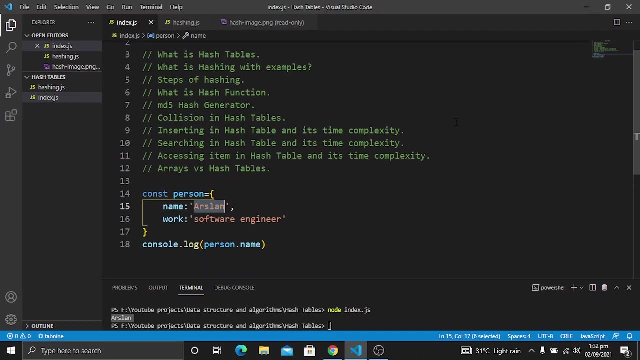 information with the help of this key which is personname. so i'm getting the name which is arslan, which is in here. so these keys are very helpful to find the certain information. so if you want to insert something to this hash table now, you want to get an, 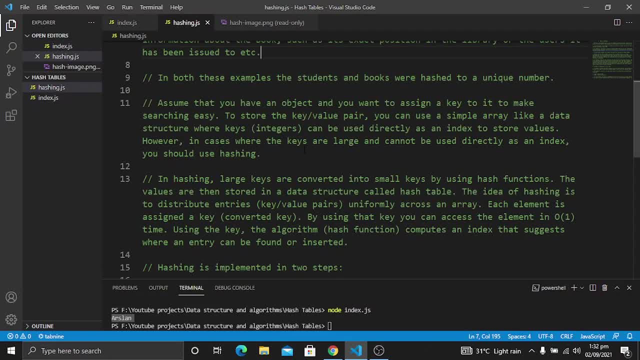 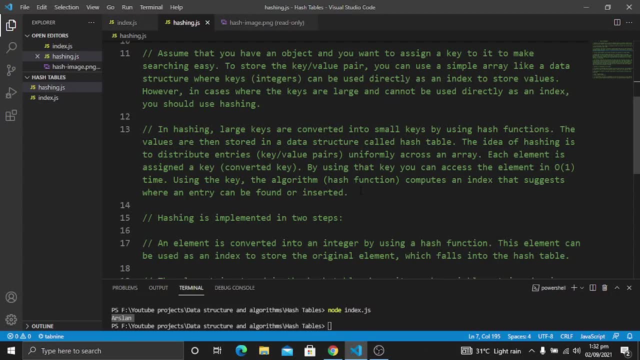 information. this key keys are very important. now the next step is going to be how the process of hashing works. how hashing works. so, in hashing, large keys are converted into small keys by using hash functions. so basically what happens in the hashing is that the large case, the large keys, are we stored in. 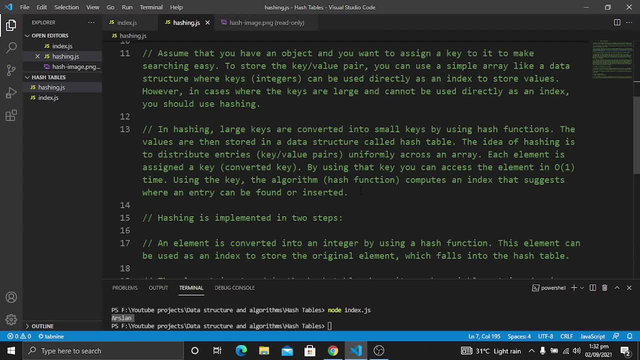 hash table, such as key values pair. so the large keys, uh, usually convert into small keys by using the hash functions. we will learn about the hash function in the next step. how, what does hash functions do? how can they convert it into small keys? so the values are then. 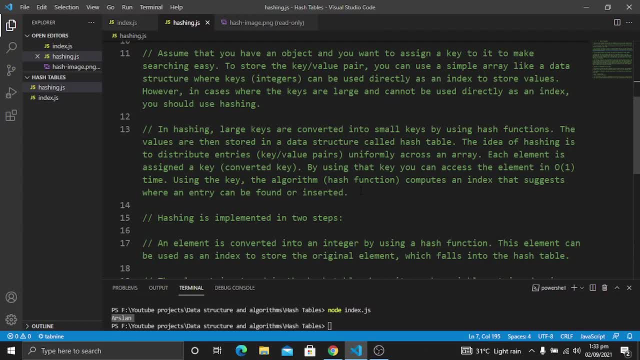 stored in a data structure called hash table. so the values, uh, that are associated with these keys. so these keys are converted into the specific memory locations, uh, in our memory, or we can say, with the, they convert into some kind of integers or indexes and in these indexes, the values, 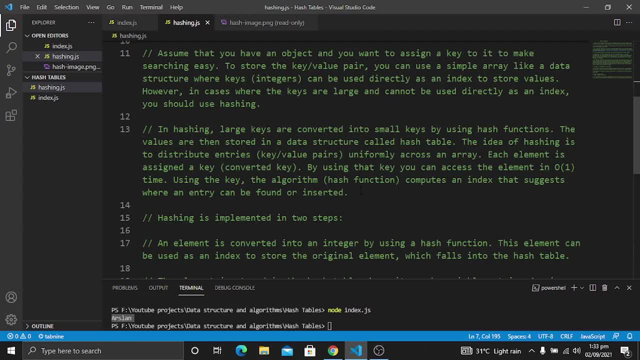 associated with these keys are also stored, so we can, if we want to get some value, we can easily get with the help of that key. so the idea of hashing is to distribute key value pairs uniformly across an array. each element is assigned a key. by using that key, you can access the 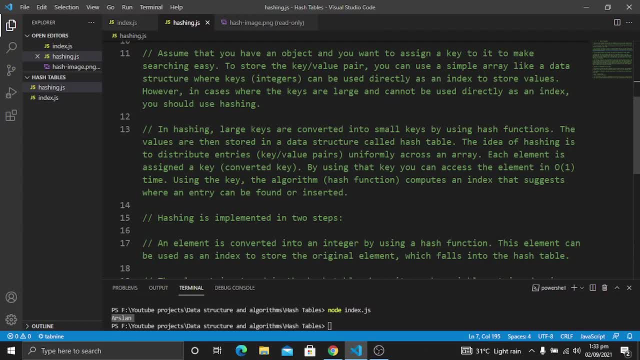 element in of one time. so this is the uh same thing that i have. uh tell you earlier that each element is assigned a key. so if you want to get some information about uh in the hash table, you have a key so you can easily get an information with the. 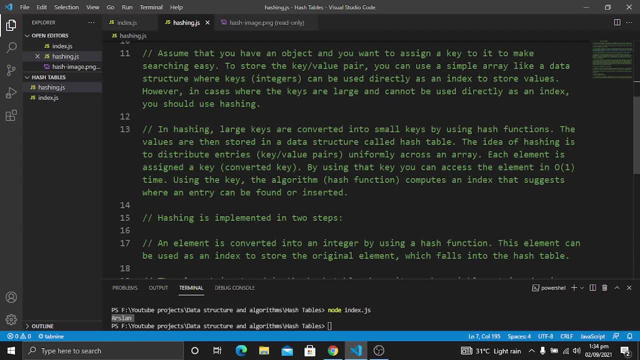 time complexity of of one, which is the constant time complexity using what we can say, using the key. the algorithm, or we can say the hash function computes an index that suggests where an entry can be found or inserted. so this is a very important line. so, for example, here is a key. 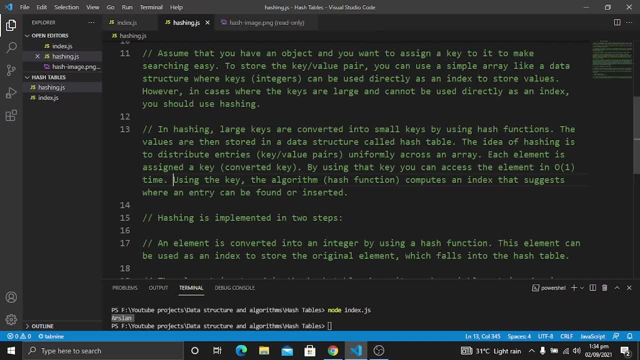 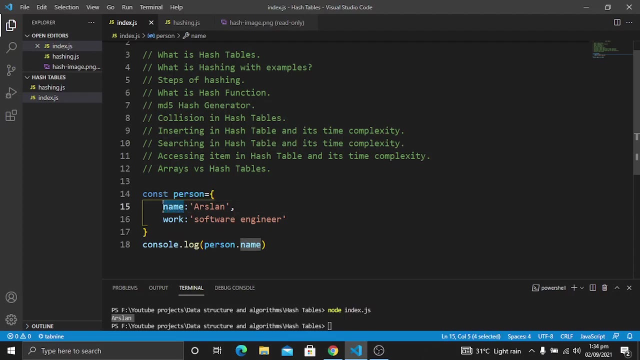 for example, name is a key. now what this algorithm, or we can say has hash function, will do? so this hash function will convert into an index something, something like so in the memory. it will not be stored as a name in the memory location, so it will have some index, some it will it. 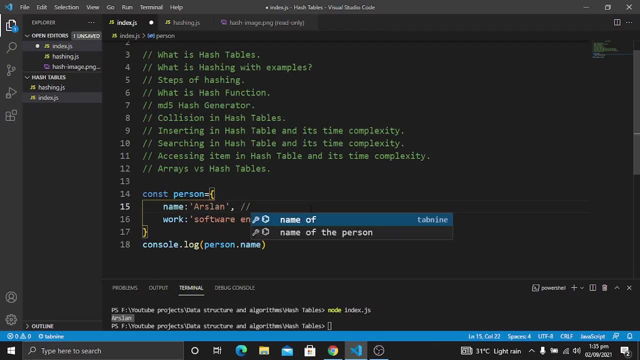 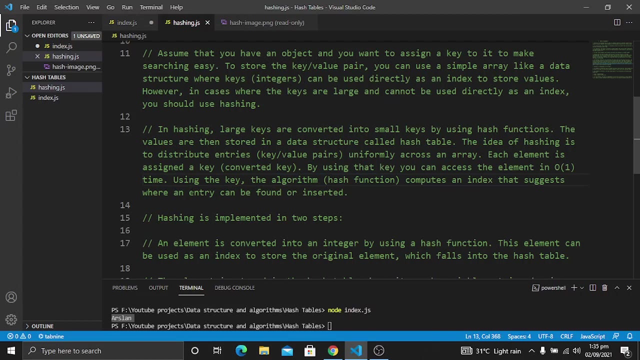 will be some oops I will write here. so it will be some random index in the memory where this value will be stored. so this will be done with the help of this algorithm, which will be the hash function where an entry can be found or inserted. so in this way we can also insert new items in the hash table or we 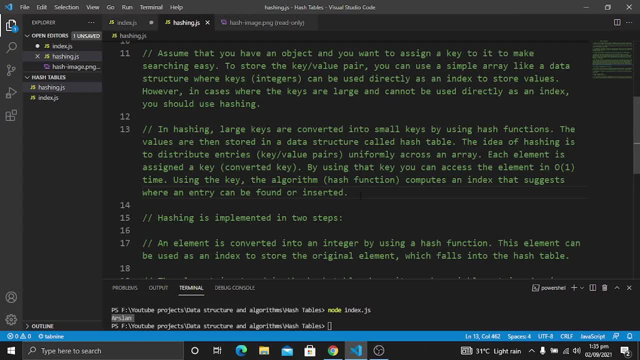 can also find the existing items in the hash table with the help of these, or we can say, the keys that we have in our hash tables or in objects. now we have learned about the hashing. what is hashing, how it is performed, what is the concept behind the hashing and why do we do hashing. so the next step is or: 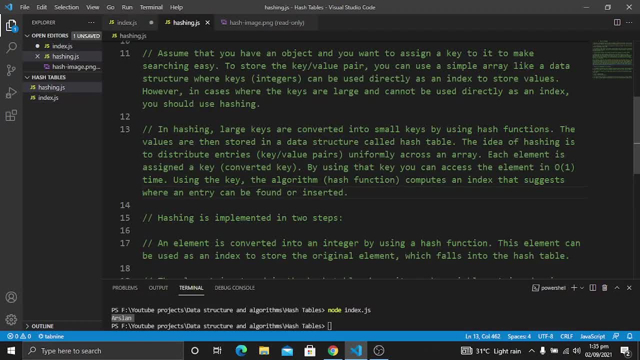 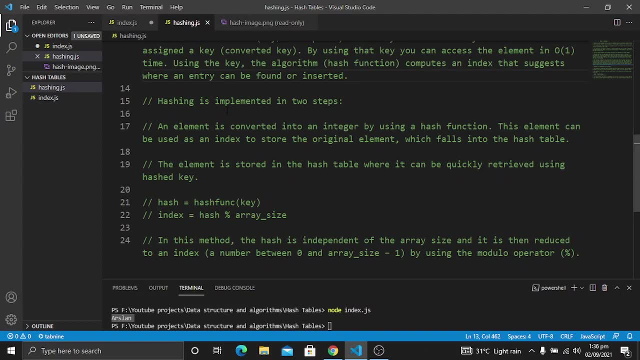 we can say steps of hashing. so how many steps hashing is done. so hashing is implemented in two steps. an element is converted into an integer by using a hash function, so the element, or we can say the keys, are converted into integer by using the. this is going to be the first step. so in this line, or we: 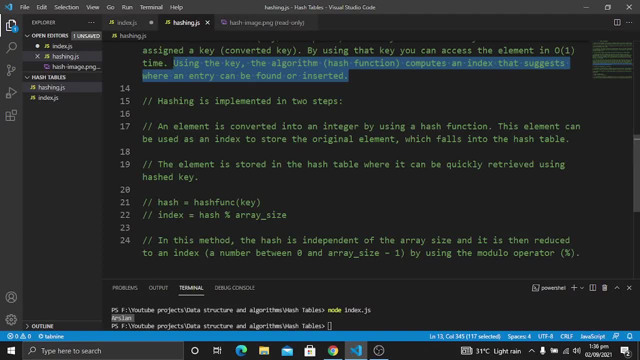 can say in this we have learned that hash functions convert the keys into an integer. so this process has will complete in two steps. so the first step is that the element, or we can say the key, is converted into an integer by using a hash function. this element can be used as an index to store the 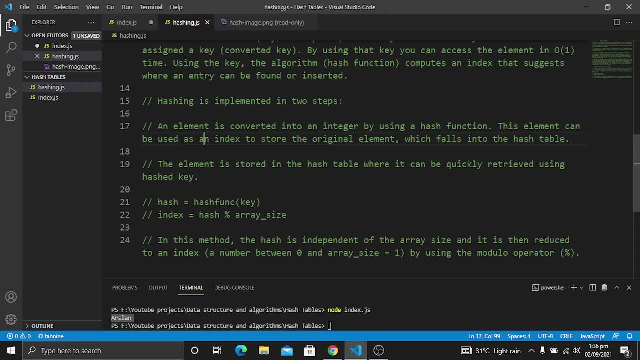 original element which falls into the hash tables. so this element can also be used as an index to store the original elements which will be fall into the hash table. so this is going to be the first step. now the next step is going to be: for example, the element is stored in the hash table, where it can be. 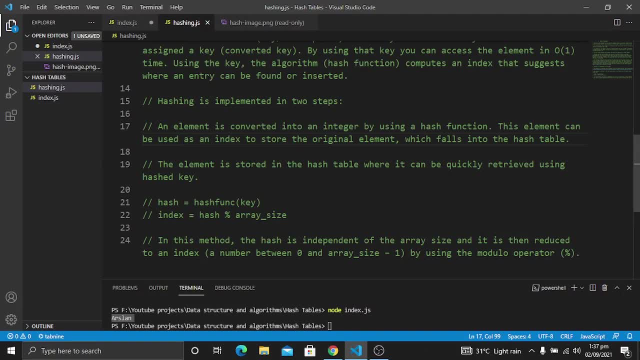 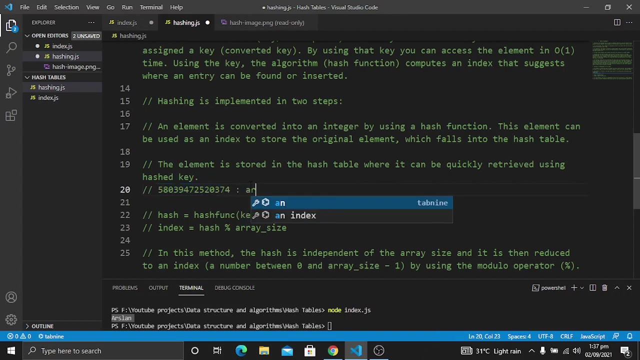 quickly retrieved using hashed key. so, for example, let's see if the element is stored in the hash table but you the certain type of key which will be something. let's see it will be this and the value stored here are something, the name, which is Arsalan. so if you want to, 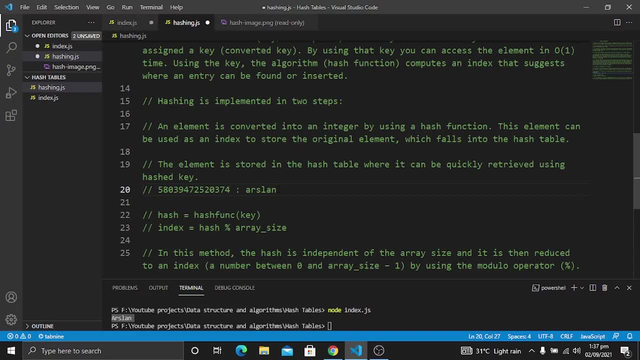 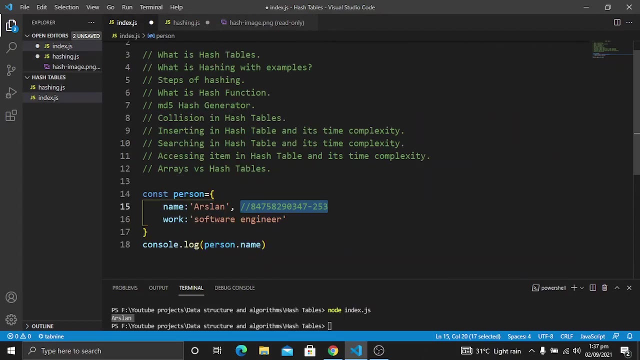 get this name. what we will do is we will have with this, or we can say this hashed key, so this, this hashed key, will have a key name of name, for example, in the data, or we can say here in the object, and this name will be converted to this. 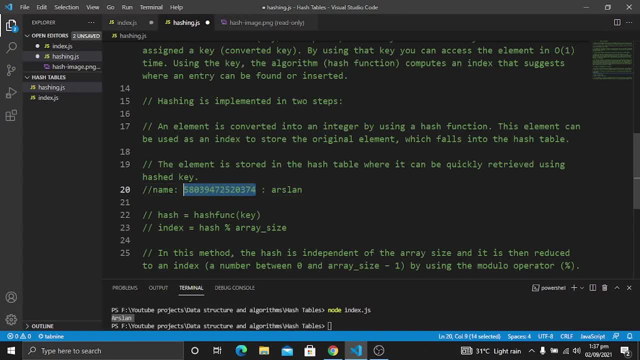 hashed key. so then we will get the information, or we can say we use person dot name here, so we have console dot log, person dot name. what it will happen is it will associated with this hashed value, or can say the hashed key, so in the memory it will retrieve the data that is associated with this hashed key. 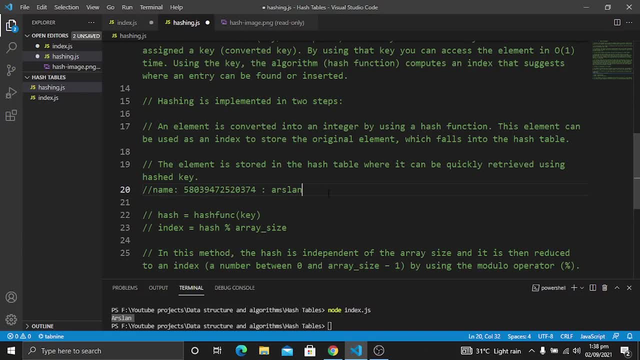 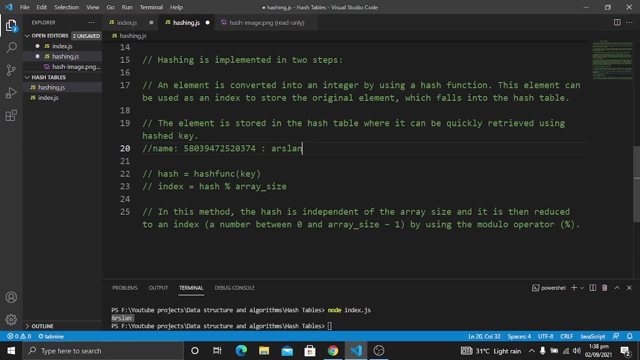 so in this way we can access the data. now, this is this step. so the first step, you can see, we provide the key in the hash function. then it has been hashed. next, what we'll do is we can use hash module array dot size. in this way we can. 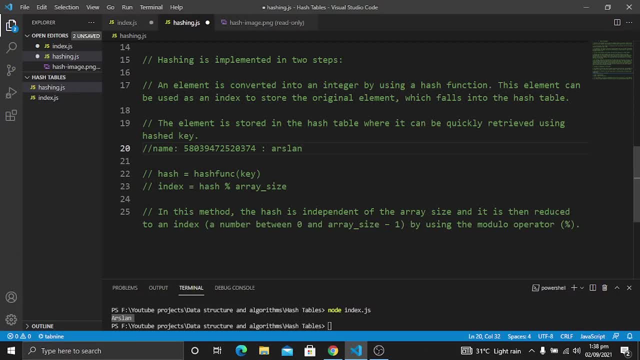 get the index in these two steps. so in this method the hash is independent of the array size and it is then reduced to an index, a number between 0 and array dot size, array size minus 1, which will be the length of an array for. so for: 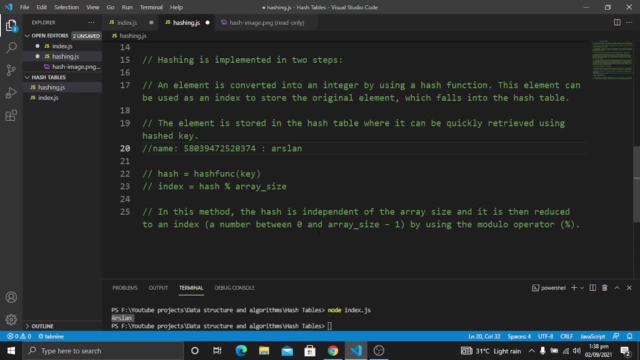 example, the number will be. for example, if the length of an array is 15, the number will be from 0 to 15 or 1 to 15 by using the module operator. so these are the steps of hashing, how hashing is done. now we have learned about the hashing, so let's move towards the next step. so 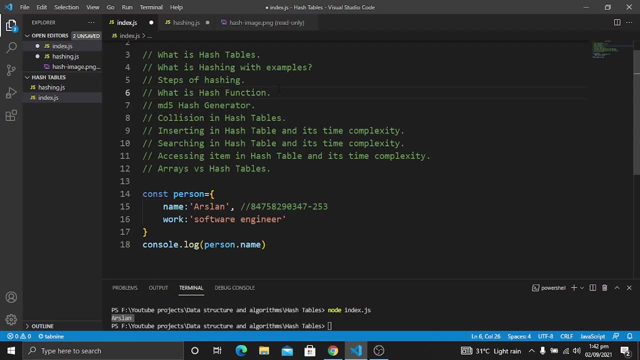 now the next step is going to be the what is hash function. so hash function is basically simply a function that generates a value of fixed length for each input it gets. so, basically, when we will provide a value, so I will go to this file in the hashing. so let's see, this is the hash function. so what this? 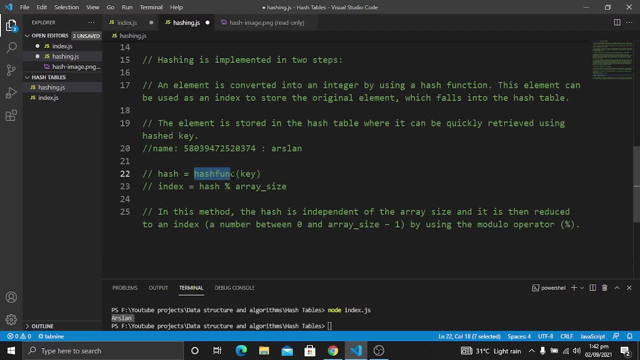 does this hash function will do? it will generate a value of fixed length for every input it gets. so, for example, here I will provide the key. so, for example, the key is going to be this name, the person dot name, and when we will provide this key to this hash function, it will generate a hash. so this hash will be some: 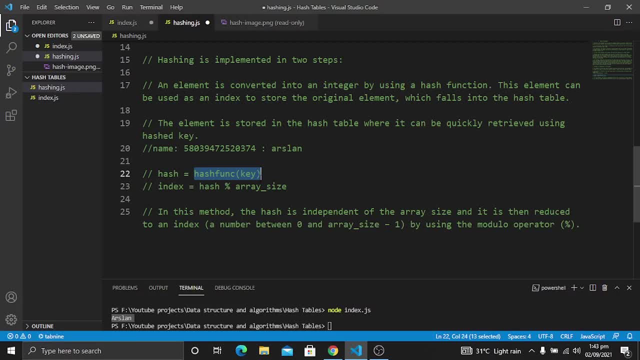 random number, or we can say of its length, which will be associated with this key. so this is the idea, or we can say this is the idea behind the hash functions. so this is the work that hash function will do. so, in the next step we have to do is md5 hash generator. 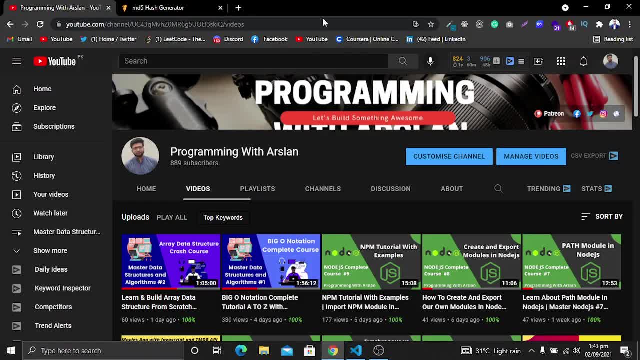 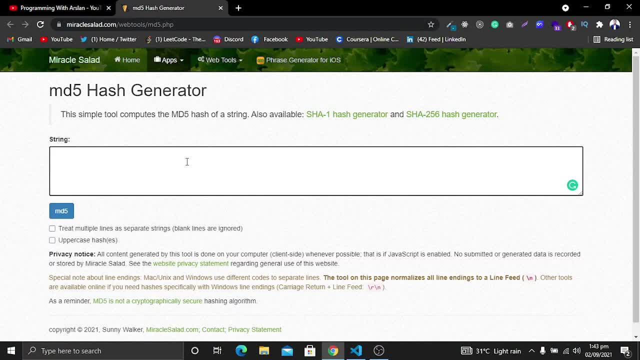 so you will learn it here that what are hash functions. so let's move here. so this is the website that I will use to explain you about the hash functions. md5 hash generator. so this simple tool can be used to explain you about the hash functions- md5 hash generator. so this: 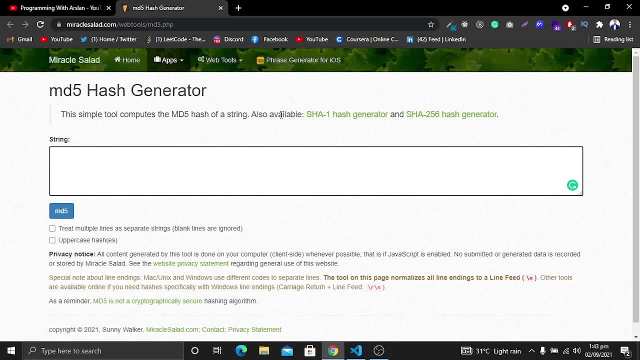 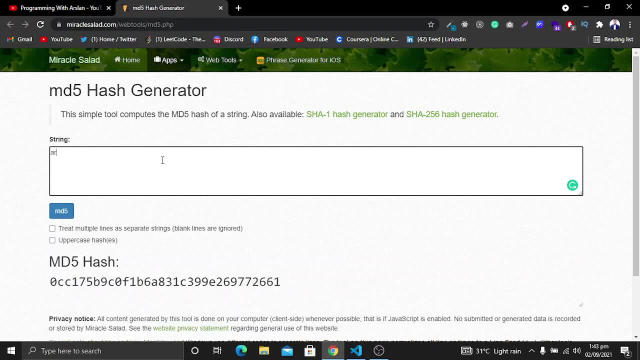 simple tool can be used to explain you about the hash functions: md5 hash generator. so this includes the md5 hash of a string also available, these. so we will use md5. so, for example, let's say, I will give it some string, so, for example, I am giving it. 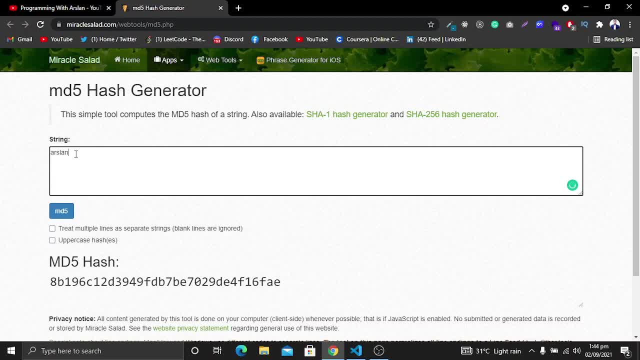 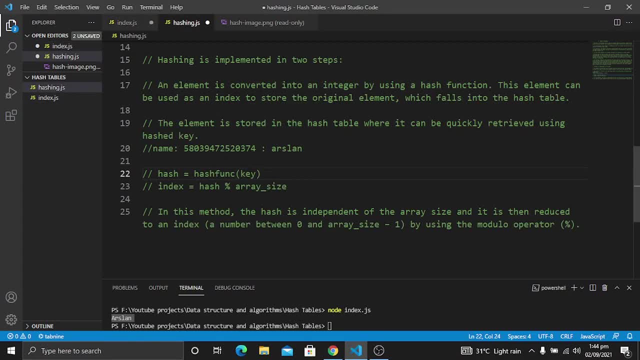 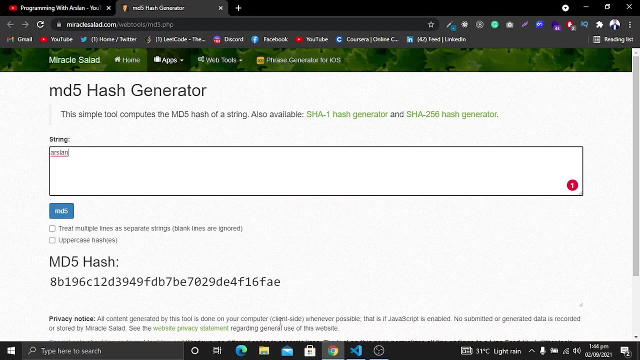 the name of Arslan. now you will see it has converted this string, or we can say here: the key oops. in this way, the key that I'm passing as an argument to this function it is being: it has been converted into an hash, so this is the. 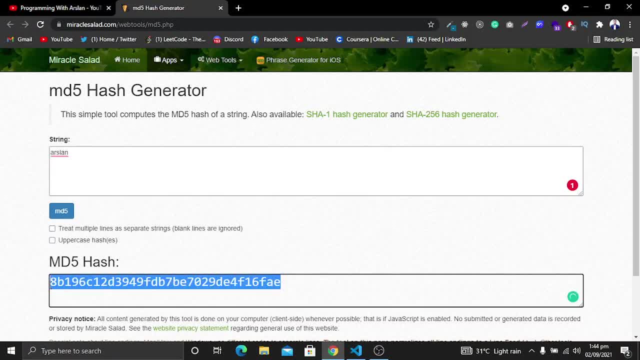 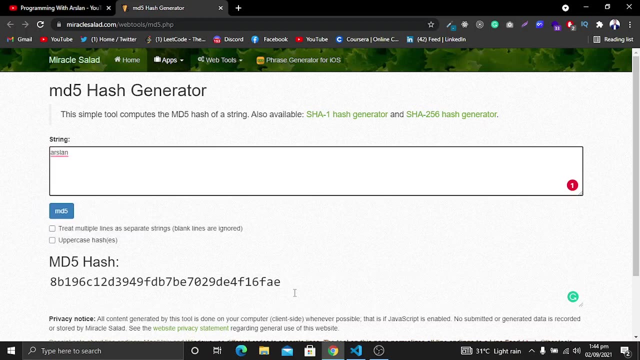 hash to which it has been converted. so I think now you can clearly visualize how hashing will be done with the help of the hash function. so this key, or we can say this key, is associated with this, or we can say this hash is associated with this key. so whenever you will write this key, you will get this edge. for example, 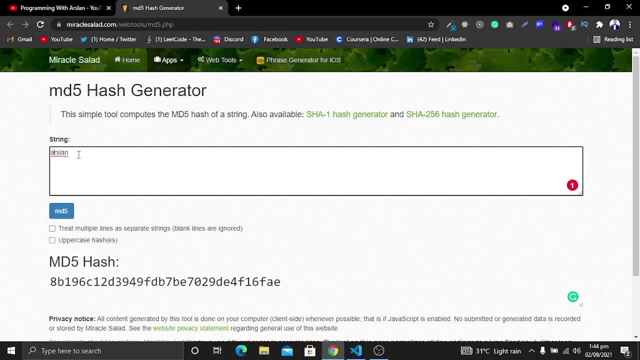 if I will simply change- or we can say convert it into the uppercase, this hash will be changed. so, for example, when I will remove a, you will see the hash has been changed completely, and when we will use a, the hash will be different. but when I will use smaller a, the hash will be the same for this key. so whenever you 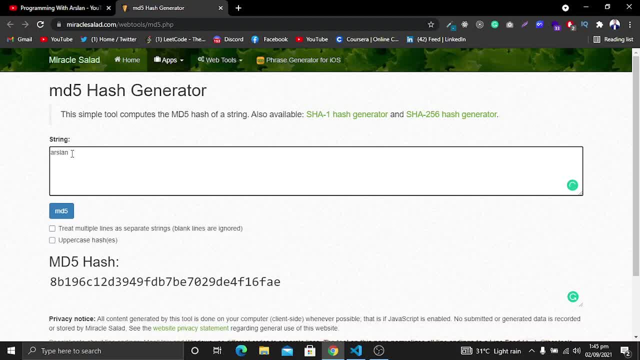 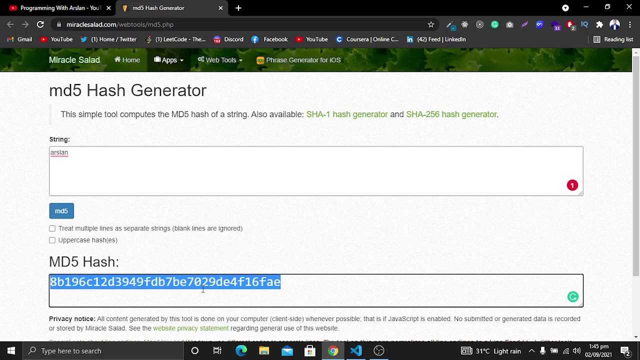 will type this key, the hash will be same. so if I give someone this random pattern, they don't have any idea of what's the input. so whenever I will give someone the idea, or we can say this, this hash, they simply don't have any idea what is associated with this. 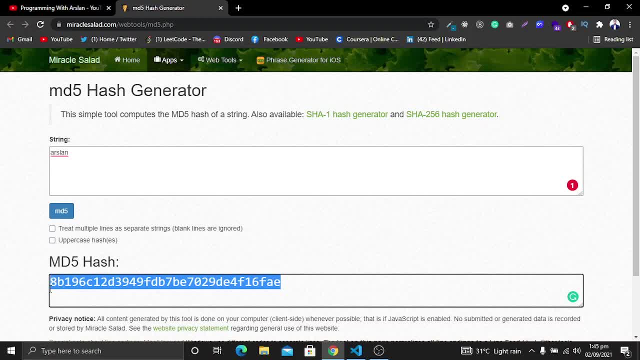 hash so you can. with this pattern you don't understood what is happening, or we can say which value is associated with it. we can get really fast data access with this, or by using hash functions. or we can say: by using this technique, we can get a really fast data access. hash tables exist in all languages, in your. 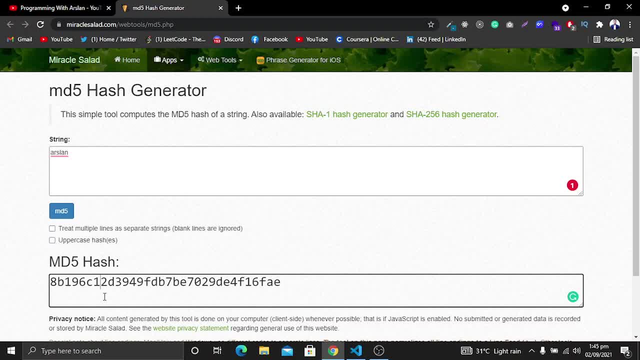 language it will have some different name. for example, in JavaScript they are objects, in Python, their dictionaries and similarly, in different languages. they have different names, but the main concept or the idea behind them are same. so this is the idea that I'm teaching you now. because of this purpose, hash. 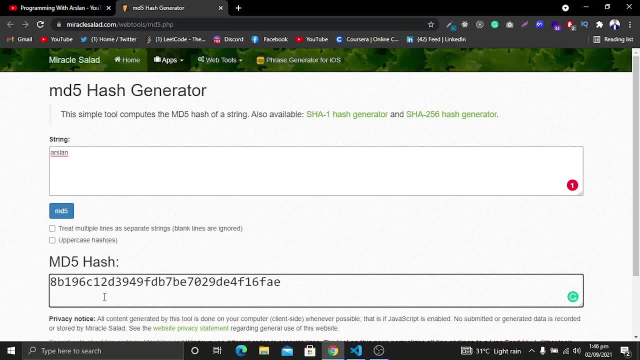 tables are used in, we can say, databases. so the work related to hash tables, for example, insert and accessing, are really fast. so this is the idea behind the hash functions or hash generator or hashing. now let's move towards the next step. so the next step is going to be the collision in hash tables. 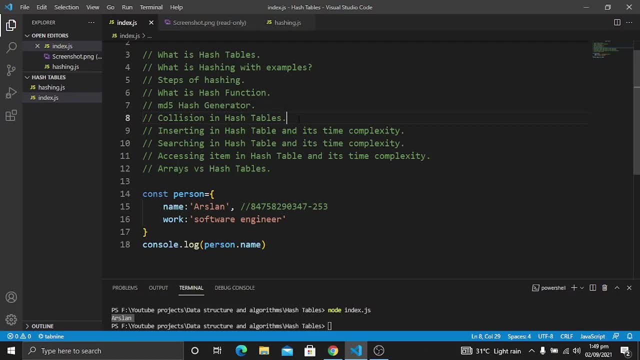 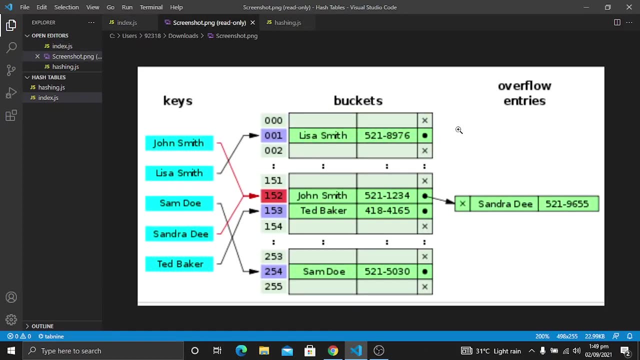 so what is collision in hash tables? so I think you will understand it better when you will visually see this. so I have a diagram for this. so this diagram is taken from Wikipedia website about the hash tables. so here you will see, we have names as keys and we have numbers of these persons as values. 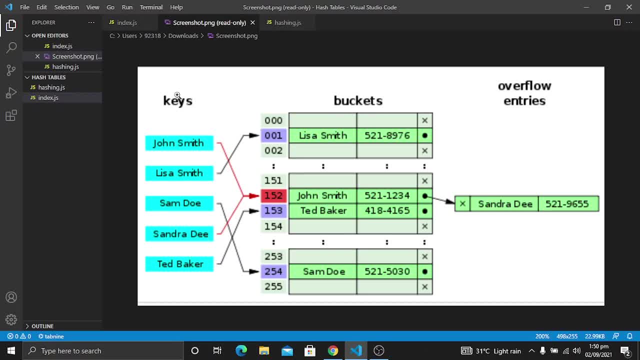 so we are storing in these buckets. so all now you will see the key. John Smith has been stored at index, at memory location. you can say 152, then Lisa Smith is stored at 001, then Sam Doe is stored at 245, then Sandra Doe is again stored. 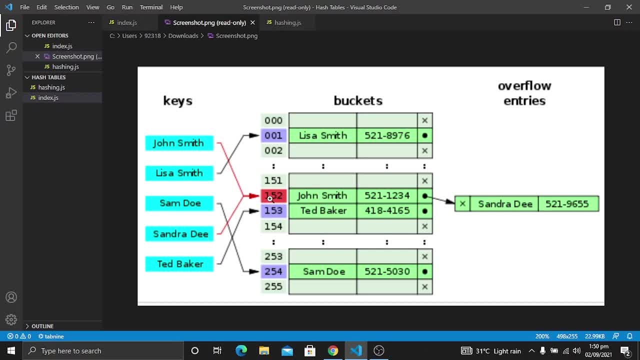 at the same index or the same memory location at 152. so this is the collision in hash tables. so, as you can see, both of these keys has been stored at the same memory location. so this is collision. so as you can see, the key with the name of the John Smith and the key with the name of the 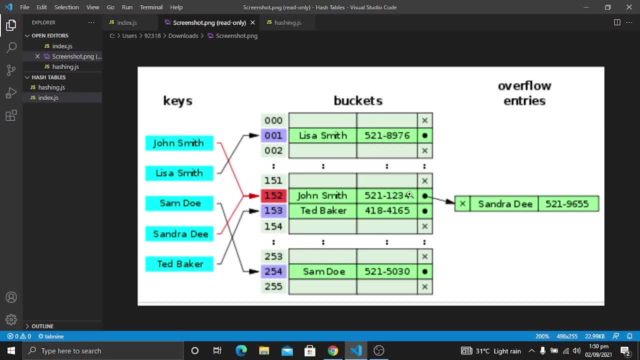 Sandra Jo is stored at the same memory location, and then there is some node, or you can say some reference to another memory location, and here this Sandra Jo and this her phone number has been stored. so, as you can see, this is the collision. when? what does hash tables or hash function do? 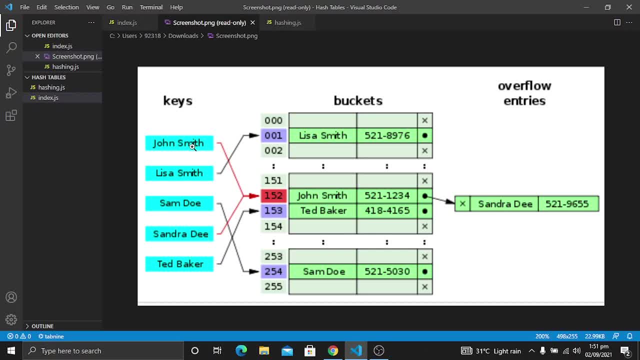 they generate or you can say they allocate the same memory location to different keys. so the this thing that you can see here, the linked list, we will learn about completely about the linked list in a detailed lecture which will become in the later videos, in the next, which will be the next, or the next two to three days. 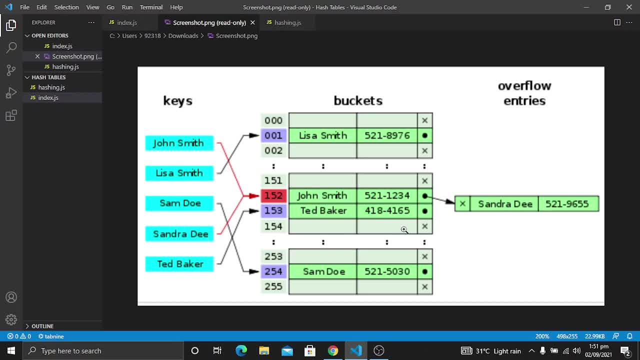 so in this, on this lecture, which will be specific about the linked list, how linked list? what is the idea behind the links linked list, What are their pros and what are the benefits. So when you will learn about the linked list, you will clearly see what will be happen here. 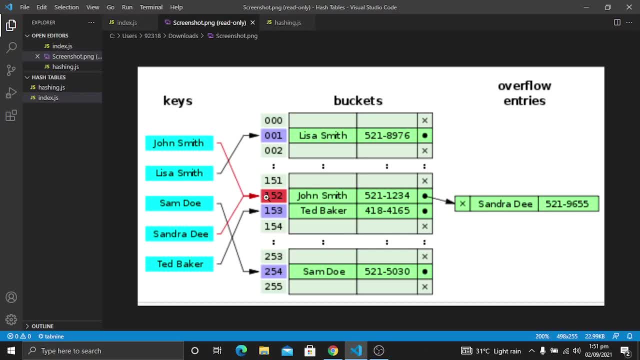 So we use linked list to resolve this issue. So the issue, which is the same- memory allocation for different keys- we use linked list to store the, or we can say to resolve this issue. There are different ways to resolve this issue, which are the collision in hash tables. 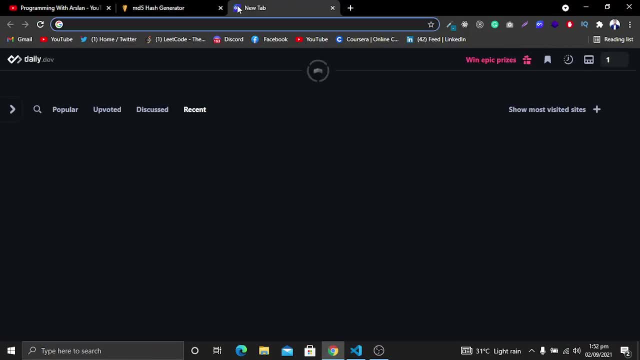 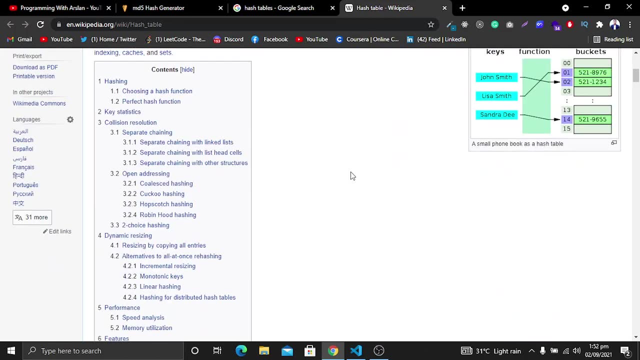 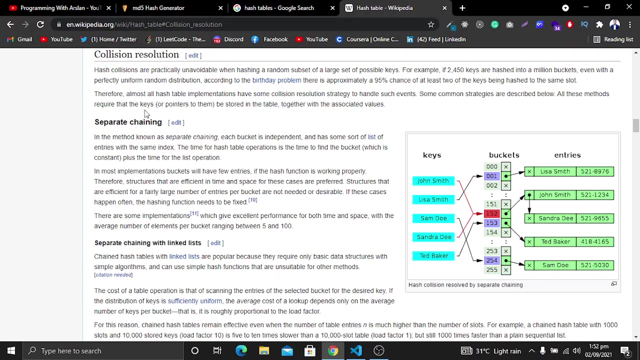 What I will recommend you to go to the- you can say Google- in the Wikipedia page. So in the Wikipedia hash tables, here you will see collision resolution. So here you will see there. These are the resolutions of this collision for, for example, separate chaining, separate chaining with linked list and separate chaining with. 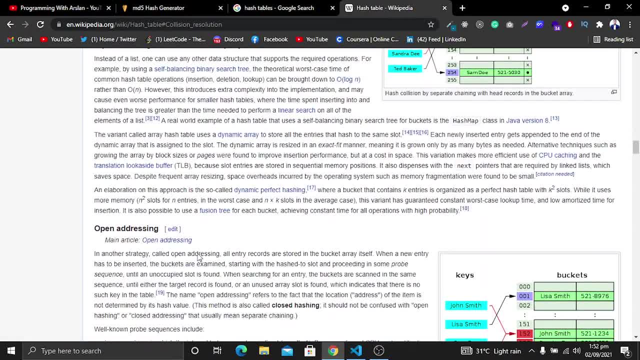 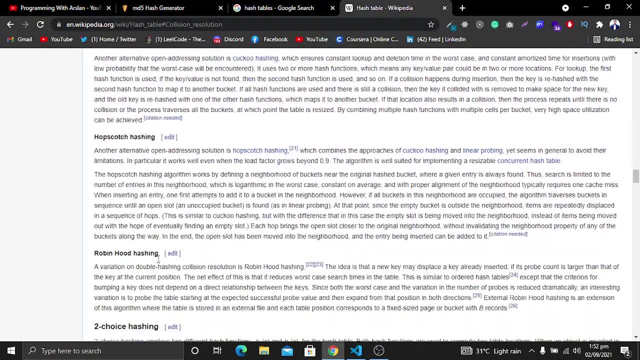 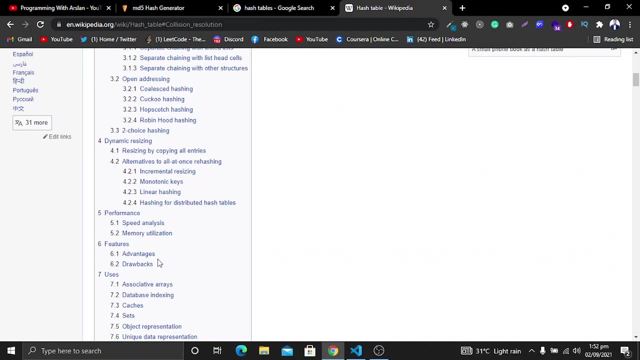 list head cells, separate chaining with other structures, open addressing. As you can see, there are different ways to resolve these issues, So I will recommend you to go to this page and, in details, read this article or read this Wikipedia page to clearly understood the hash functions. 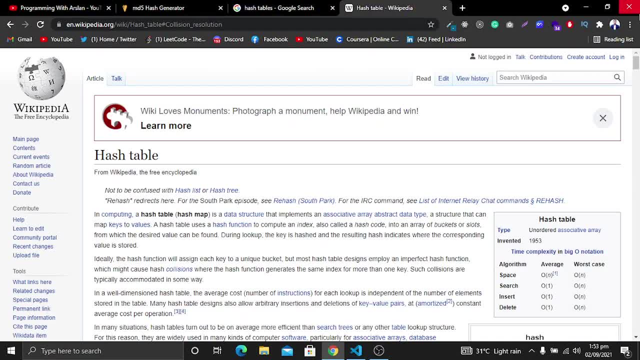 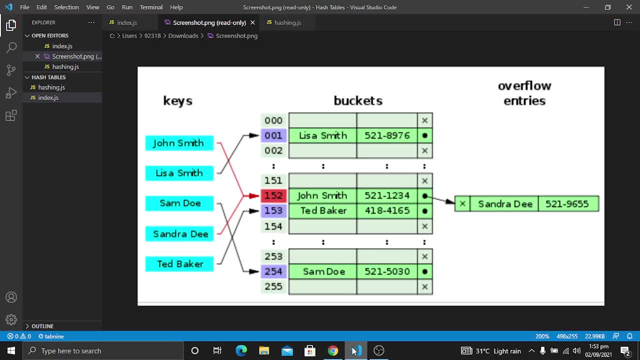 So when you will read this, you will have a clear and understanding: what are hash tables, how they work behind the scenes, how collision happens, how we can resolve these collisions, And you will cover everything in detail. So this is about the collision in hash tables. 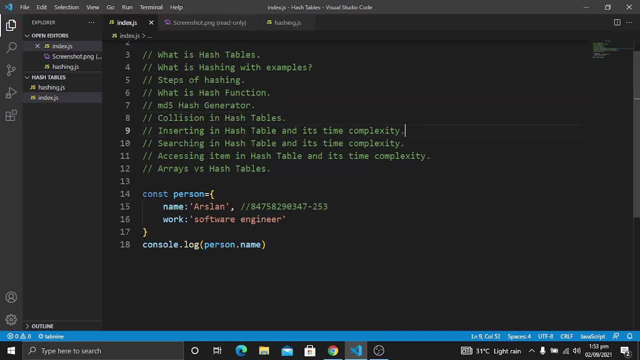 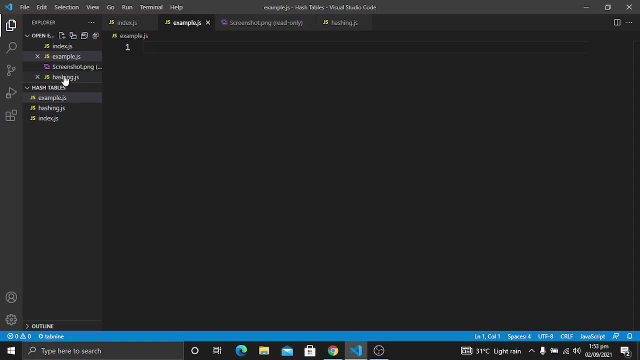 The next step is going to be inserting in hash table, and it's time, complexity, searching and accessing. we will perform this operation. So let's create a new file, So let's say, give it the name of example: dot JS. Now what I will do is I will create here a hash table. or we can say: 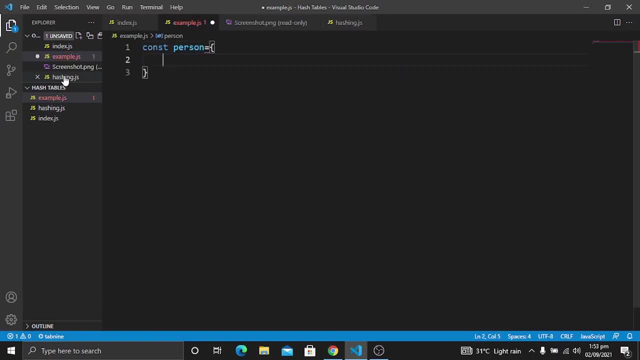 an object with the name of person. For example, I will create an object with the name of person and I will give it a name of Arsalan, and then I will give it a job. So the job will be software engineer. And then let's give it an age. 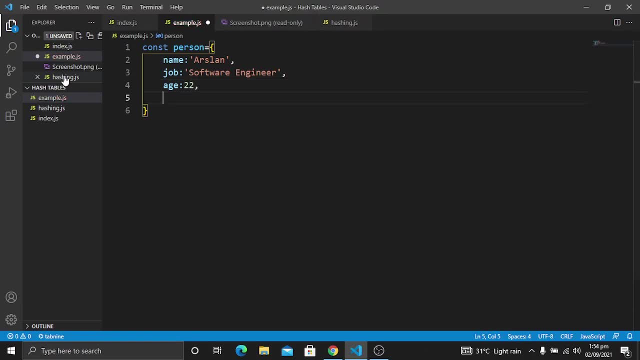 Let's give it an age of 22.. And then let's give it some work, which will be the function. So in the function we will just log it, which will be console dot. log that On YouTube tutorials. Let's save it. 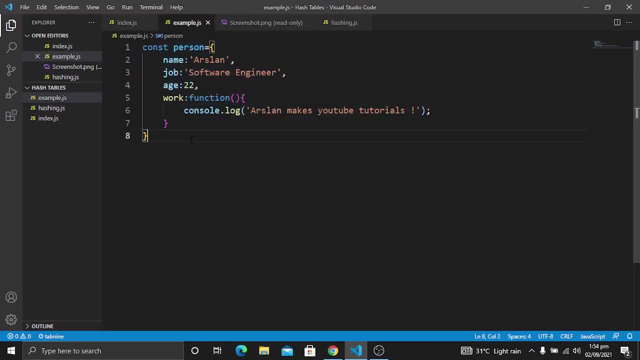 So let's see, This is the object, or the hash table or the dictionary in Python. So in JavaScript, these are the objects. we call them as objects. So let's see if I want to access something from this. So, for example, let's say if I want to access this job. 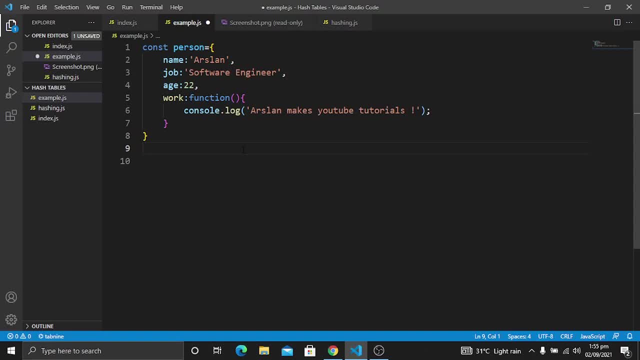 what is the job that Arsalan is doing? So, simply, what I will do is I will use console dot log and I will use person dot job. Now, you will see that when I will so clear the terminal, So run the code here. 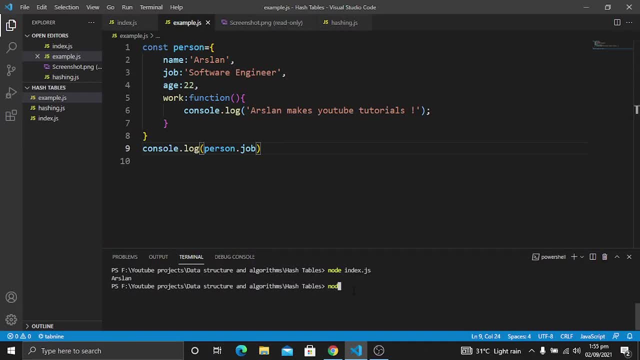 Now you will see: Oops, So this is a different file node: example: dot JS. Now you will see, we are getting software engineer. So now you see how easy it is to get an data access from the in the hash tables. Now you will see, you can now the name of the. 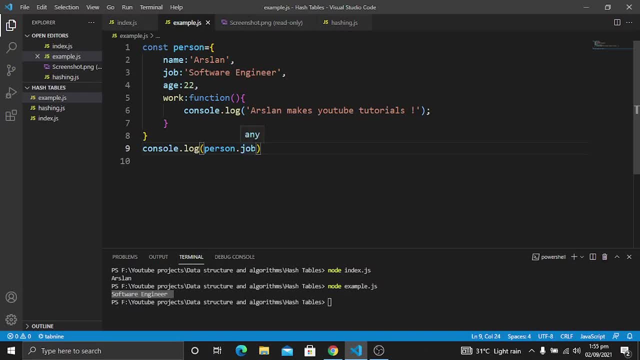 Key. you have a key and with the help of this key you can clear, you can easily and for in the foster, you can get the data access. So this has a Time complexity of one. There are no operations which are considered, However. 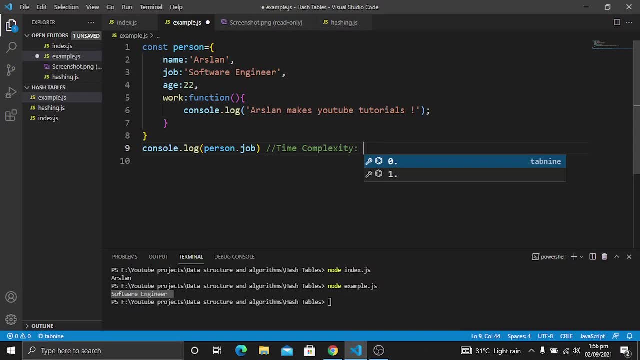 what we can say is if the length of this hash table may be hundred or thousand, You don't have any concerned about that numbers because you have a key and you have index, specific index, and add that we can say: instead of index we can say: you have a key and with the help of that key, 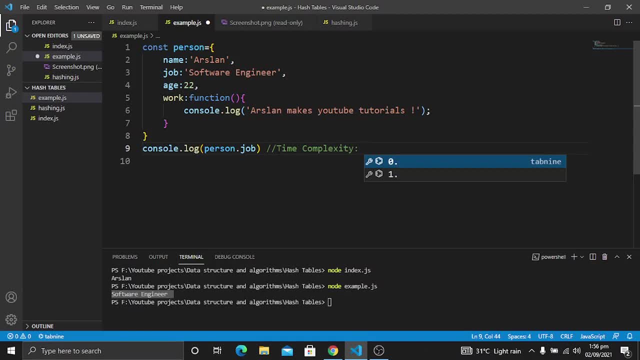 you can get the value that is associated with that key. So in this way you can get the access to the data with off one time complexity. So this is the Linear time complexity in your time complexity. Oops, not linear time complexity. 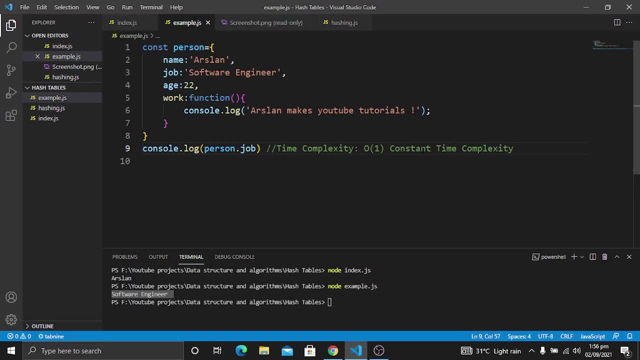 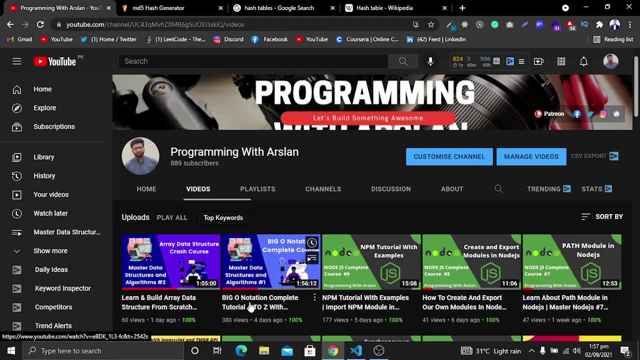 It is a constant time, Complex, Sorry for it. No, I have clearly explained in this two hours long bigger notation Complete tutorial, where I have literally explained everything: how you can calculate the big connotation, How you can simply visualize in your 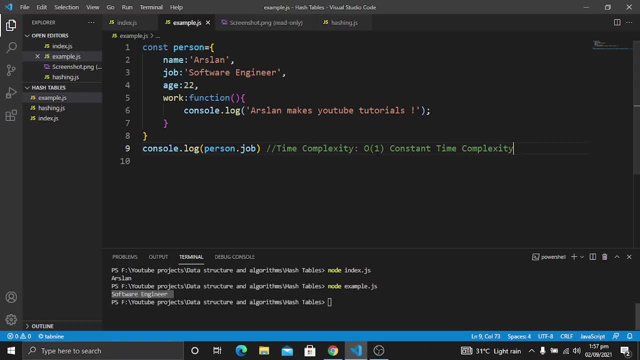 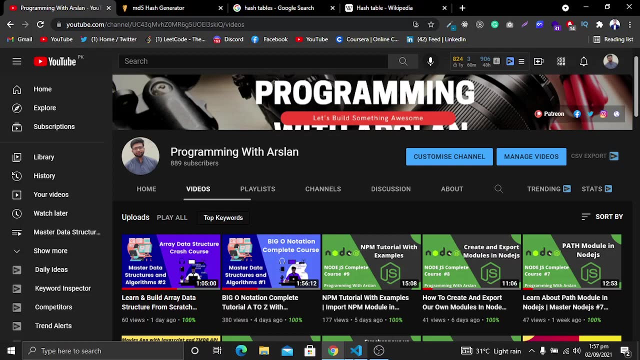 Mind that what will be the big connotation for this algorithm. So if you are confused about the big connotation, I will highly recommend you to watch this tutorial, which is about the big connotation: complete tutorial A to Z with examples in this tutorial. 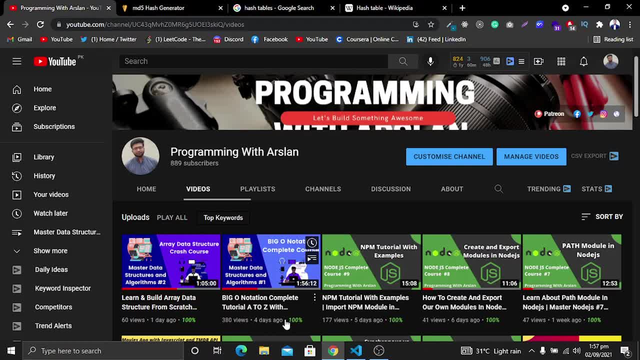 I have explained everything with the help of every concept, with the help of two or three examples. So if you are a beginner in DSCR, if you are a Into the DSA for a long time and you are just still confused about the big connotation, 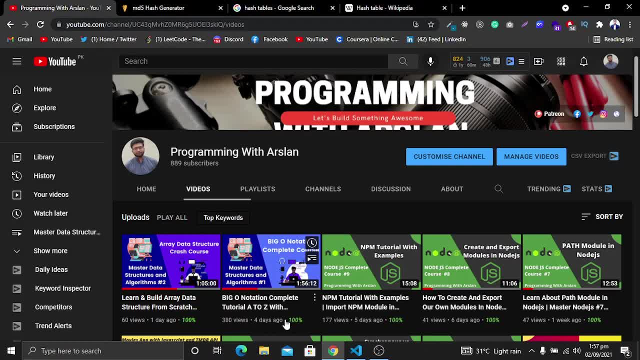 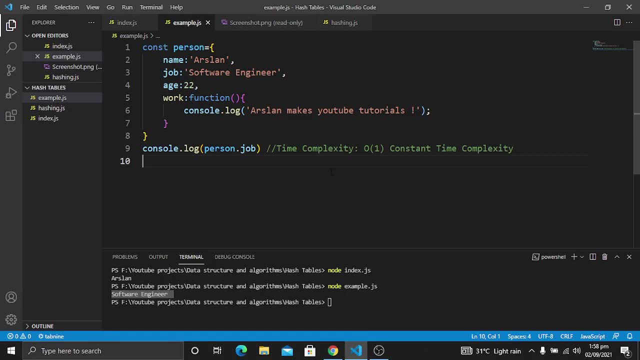 I will highly recommend you to watch this tutorial because it will clear your confusions and you clearly understood about the big connotation. How can calculate the time complexity for certain algorithm? How can we calculate the space complexity? Now, in this way, you can access the data. 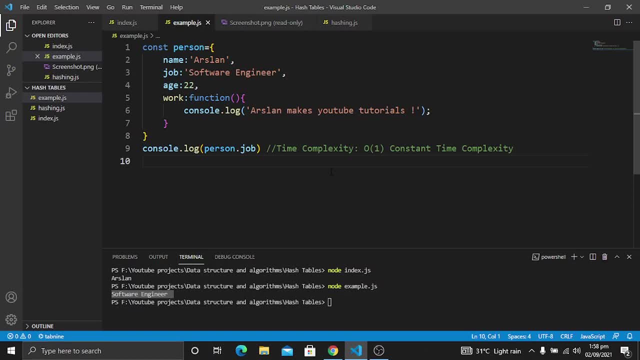 With the help of this function, or we can say, with this approach, not function with the help of this approach, because you have a key name and with the help of that key, you can easily access the data. The next thing is: let's see if we want to insert the data into the or what we can say. 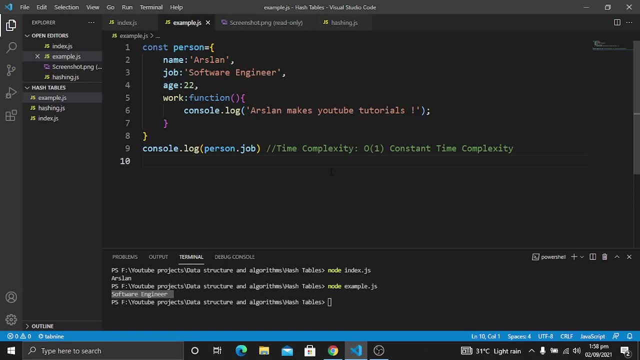 Into this hash table or object. So for this, what I will do is, let's say, if I want to add this port, This port that are sunlight, So let's see person dot sport. Next thing is here. here You can add the value that you want to add. 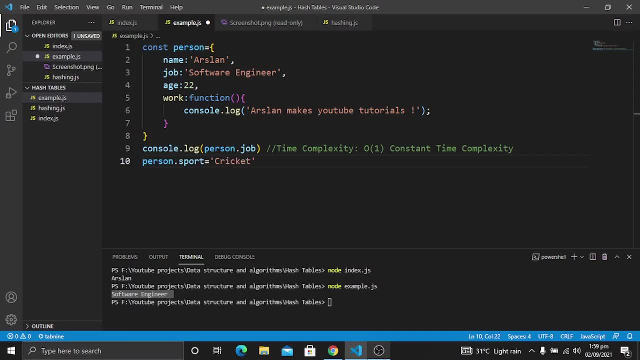 So, for example, let's say I will add the cricket, So what it will do is it will add the cricket at this position in this object. So if I will console dot log this object, so console dot log this person object, Now what I will do is: 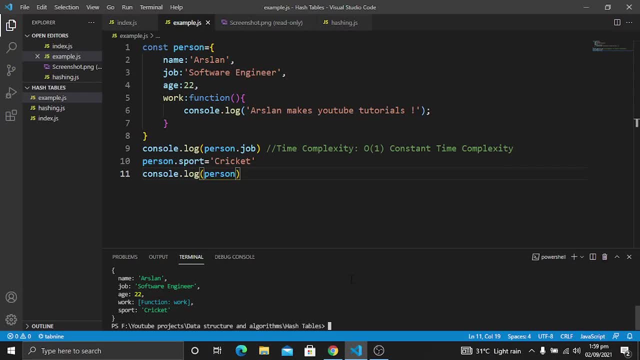 I will clear the terminal. run the code again Now you will see here clearly, see here. What is happening is We have this person object and here we have a name On job: software engineering, age 22, work. is here this function? Then we have added sport, cricket. 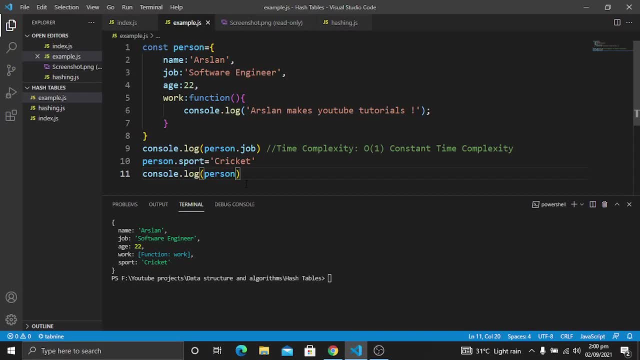 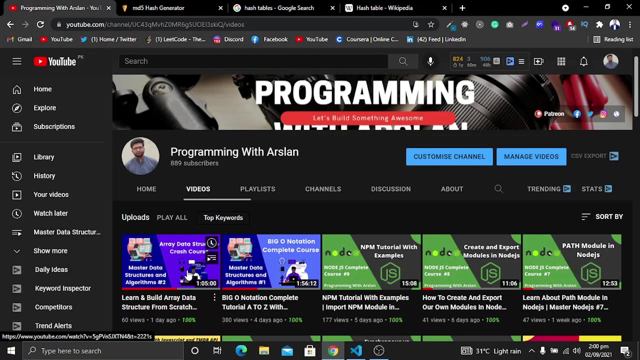 So now you will see how easy, or we can say how fast, it is to add, or we can say insert The data into the hash table. So it is completely opposite to the arrays. So in the arrays video we have discussed, discussed how expensive is it to insert the data into the arrays? 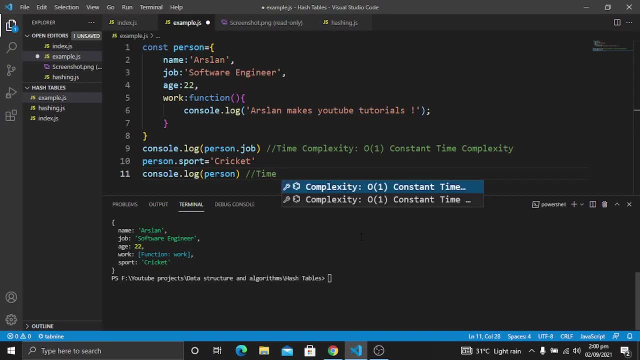 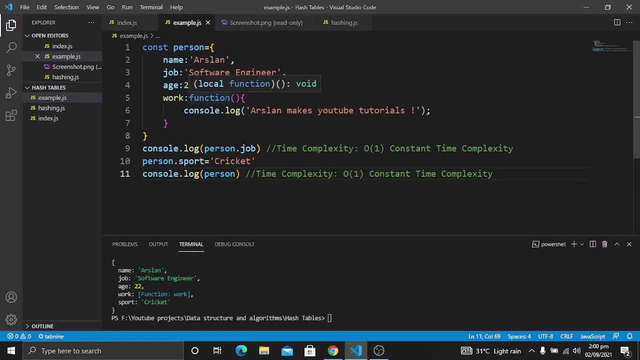 Now this function- or we can say this- will have a time complexity of all fun, which will be the constant time complexity, So it doesn't matter how long this has table will be. you have a key and you have the name of the Object. 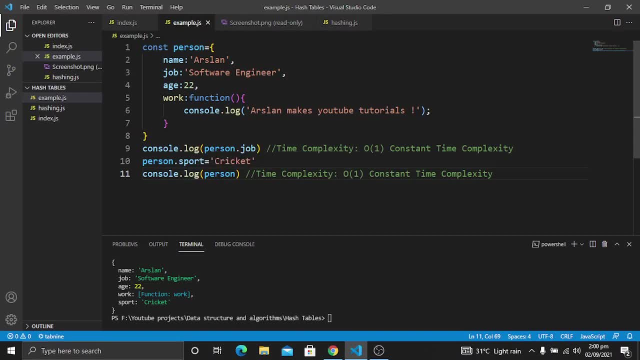 which is percent, and you can easily insert person dot sport the value into this Yep or hash table. So this is easy. Let's see We want to access first of Person dot work. So let's see, We want to search this and this object, person dot work- and we want to access this here. 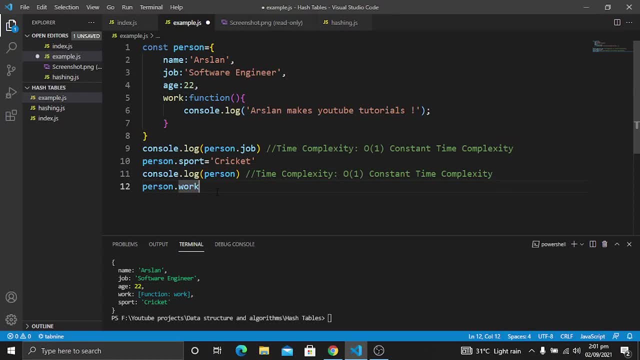 This console dot log or this function. So what I will do? I will simply Use this technique, which will be person dot work, and I will console dot log it. console dot log, Yeah, person dot work. So let's comment it. 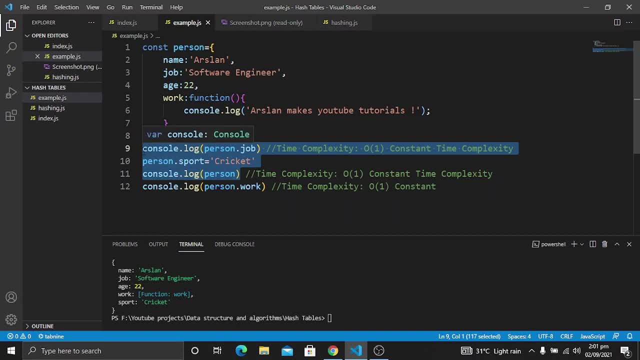 Let's remove the upper ones, So simply comment them out. Now let's clear the terminal And run the code again. Now you will see we are accessing this function, which is person dot work, simply. So let's see if we use parentheses. 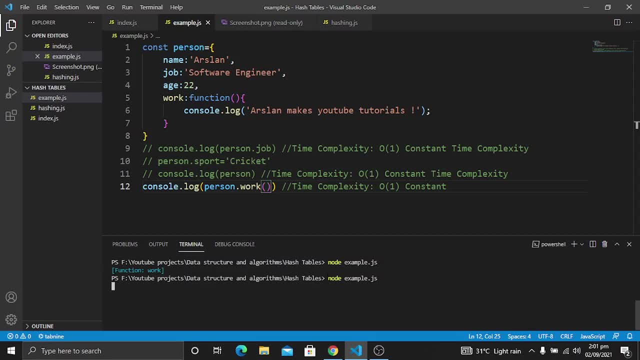 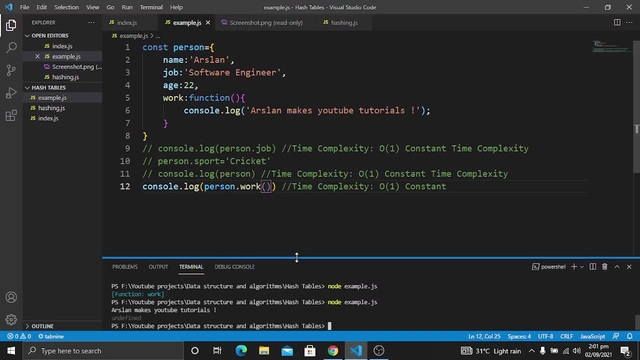 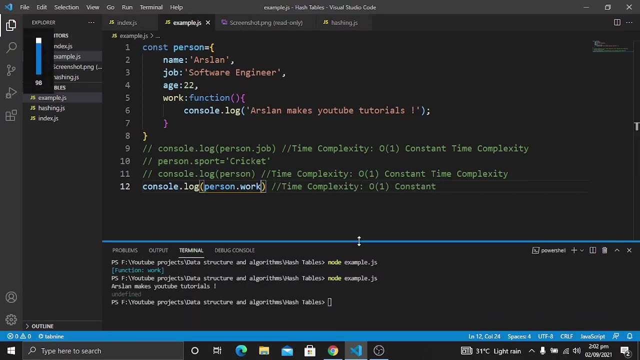 what will happen. So if we use parentheses now, you will see we are getting undefined, So we don't have any concerned about it. So we are just saying that whenever we use person dot work, we are accessing this function And we get the function. 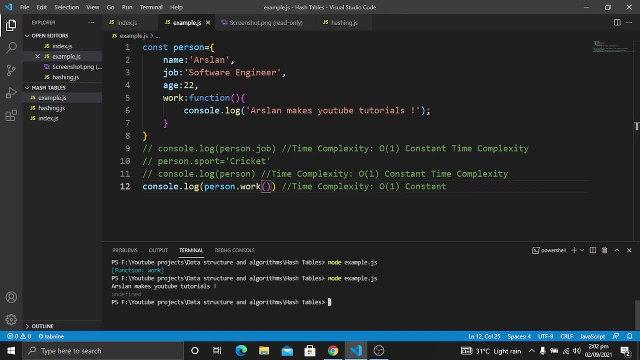 But with parentheses. what we will get is we will also get the value, For example the console dot log. here Sun makes YouTube tutorial. I'm getting this value here, So this will also have a time complexity of one. So you can see the operations are very. 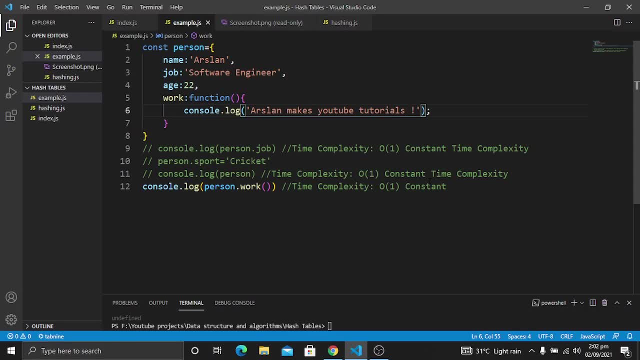 very fast in hash tables. So these are the reasons that hash tables are used in databases. Now we have learned about how can we access the data, Or move, or we can say: access the data, insert the data and what will be their time, complexities. 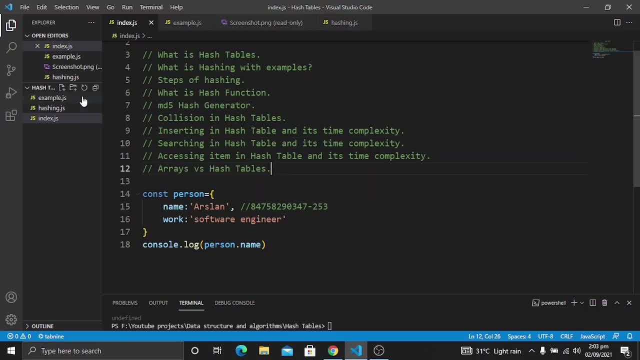 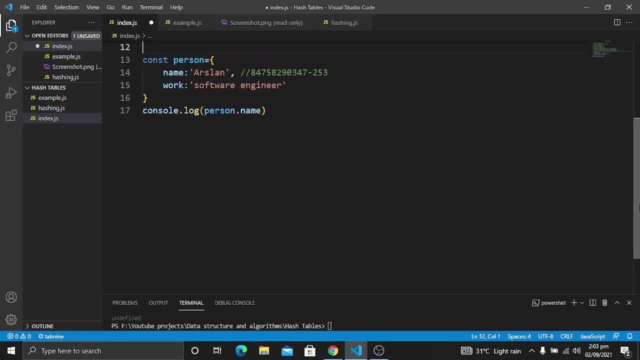 The last step is arrays versus hash tables. So let's discuss about it. So what I will do? I will remove it from here. Paste it here. Now let's see the difference between, or we can say the difference between, the hash tables. 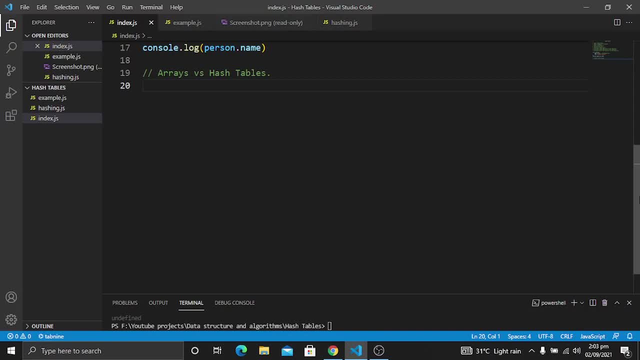 And the arrays. So the difference will be done on the basis of the operations they perform. So, for example, first of all I will write about the arrays. So in the arrays search function, So in the array search function, will have a time complexity. 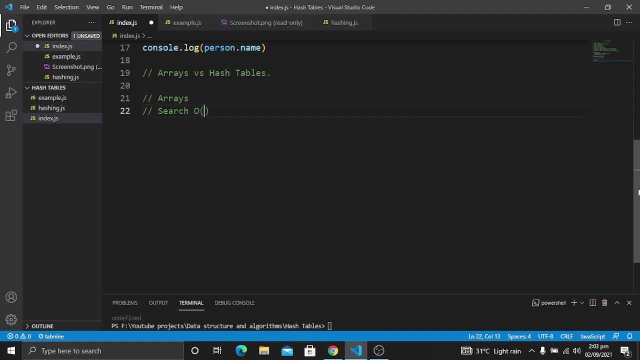 or we can say: the connotation that we can calculate is off and which will be the linear time complexity. So it will. it means that you have to loop through the array in order to find a certain element, Whereas in here I will compare them. 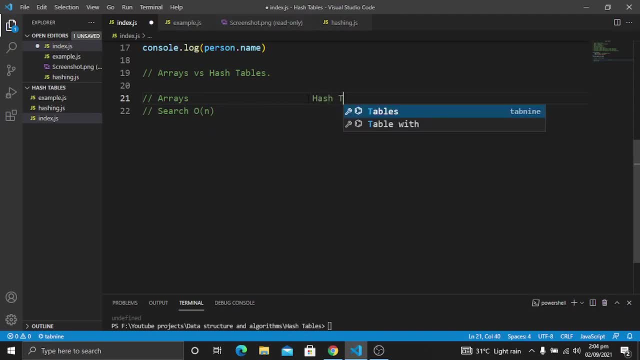 So here will be hash table hash tables. Now this searching in hash tables will have a time complexity of search of one. So this is because you already know the keys and it will be very easy for you to access the data. Or you can say the search the data in this hash tables as compared to the arrays. 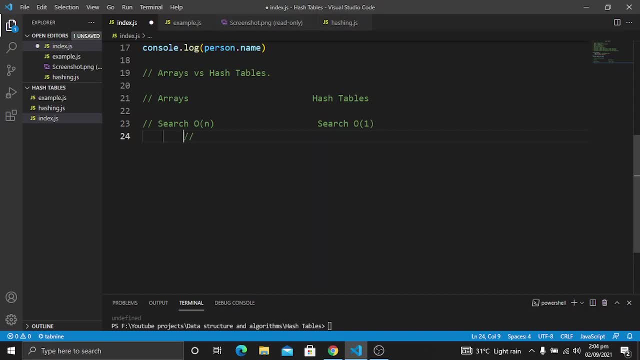 So the next operation that we want to convert, or we can say the compare, So lookup, which will be the access, So the lookup in arrays, will have a time complexity of one, because we simply have indexes in arrays and we can compare them. 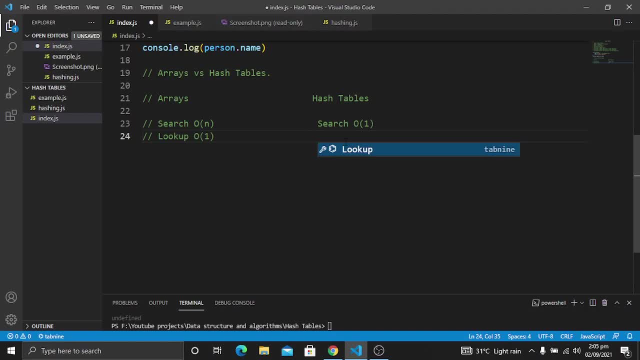 So not compare them. What we can do is we have, for example, let's say, we have an array, and in the array we have 10 items, and we want to access the item that is at the index five. So what I will do is I will simply use these techniques. 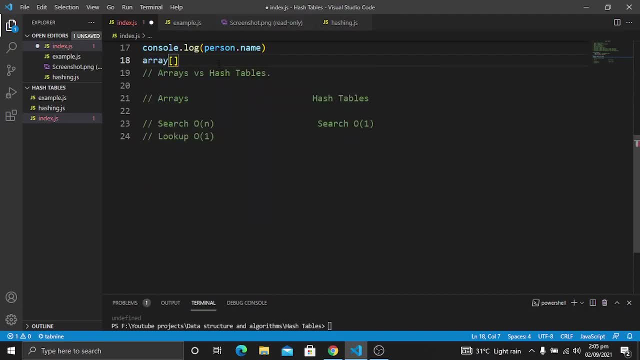 For example, if I have an array, if I want to get the value which is an index five, so I will simply use this thing, which will be in the array, I will pass the index and we will get the value, and we can store that value in something like this item. 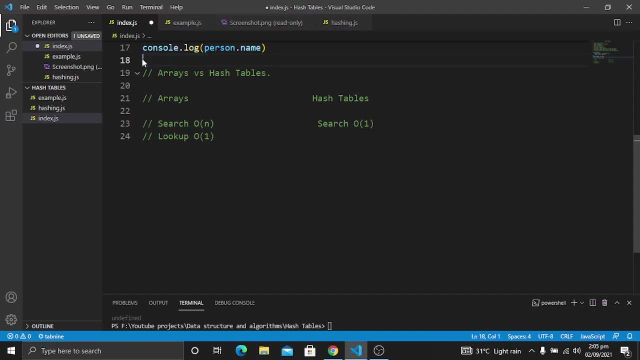 And in this way you can access the item in the array, Whereas in hash tables it will have the same complex time, complexity which will be the O of one which will be. we can access it by using the percent dot name, with the help of the keys. 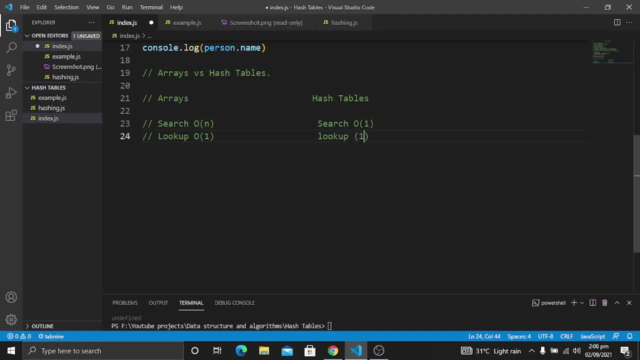 So the lookup is going to be the same, which will be the O of one which is constant time complexity. The next thing is going to be the push. The push pushing in arrays will have a time complexity of O of one which will be the constant time complexity. 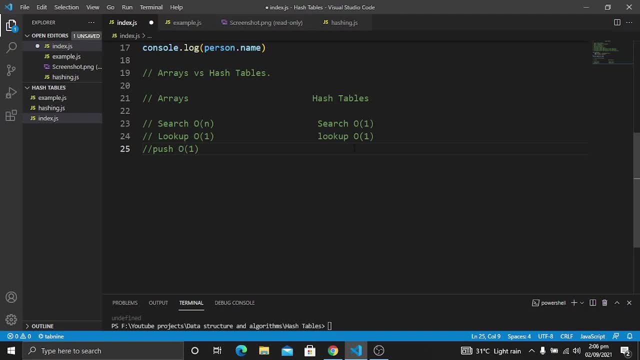 So the push means the appending. So appending means when you want to add the item at the end of an array, So it will have a time complexity of O of one. We have clearly understood in the arrays lecture that how these things are performed and how we can calculate the time complexity of it. 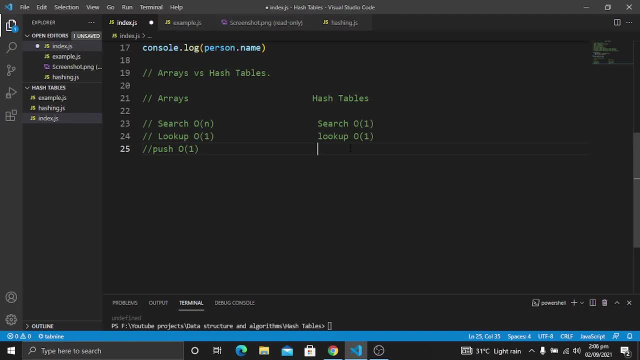 And we have clearly discussed the concepts that on the basis of which we use the push method or the append method, And we have made these push methods from scratch by using- or we can say on this tutorial in the previous lecture. So if you want to learn about these things, 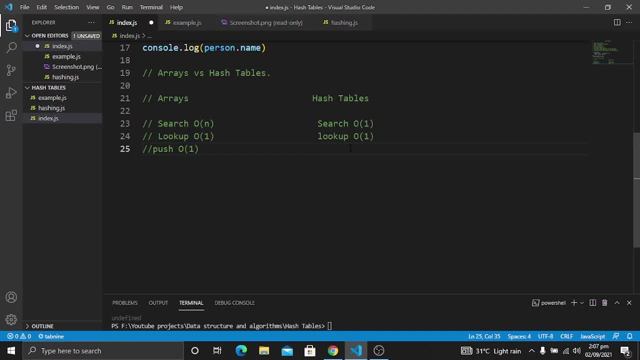 you can watch this tutorial Now, pushing in this, or we can say we'll have a time complexity of O of one and it is really fast. Then we have an insert operation and the insert operation will have a time complexity of O of one, because when you want to insert an item to an array, 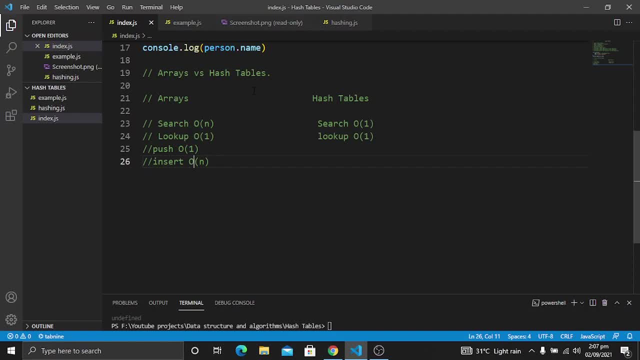 the other items that are present will be more towards the next steps or we can say the number of operations will increase if the number of items in an array is increased. I have explained it in details in this array video. Now inserting is expensive and also the searching is expensive in arrays. 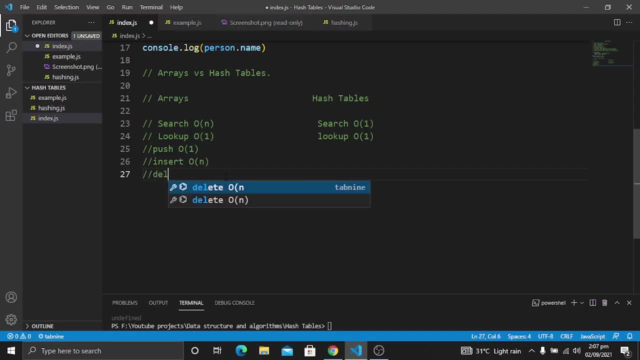 Now the next step is deletion. So deletion is also expensive in arrays. It has a time complexity of O, of N, which is linear time complexity. It means if the number of items in array increase, the number of operations will also be increased. Now let's see about the hash tables. 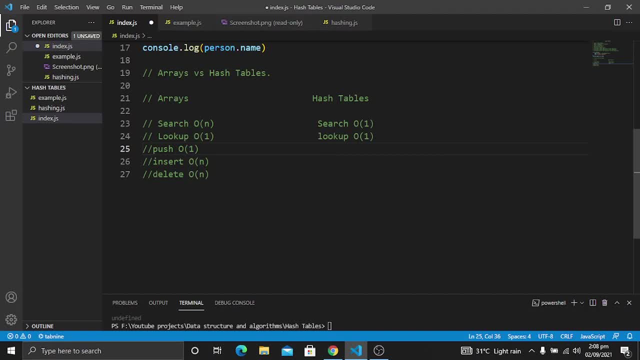 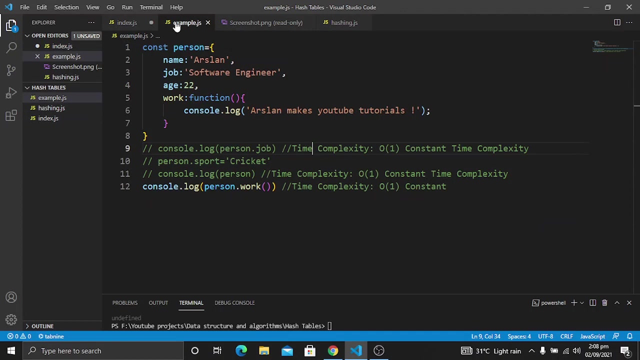 So we have looked of our research and access our lookup Now, insert for insert will have a time complexity of O, of one because it is really really fast. This is because, with the help of here, we have learned in the example that inserting is really fast. 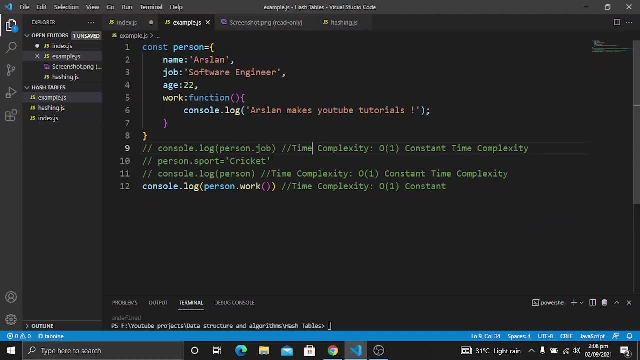 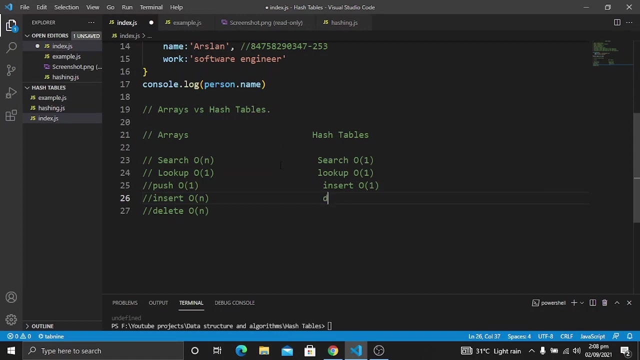 Because we can add simply by percent: dot sport cricket. with the help of case We can clearly or we can simply add the value associated with this K into the hash table. It is not concerned about the length of this object or this hash table. So inserting is not expensive here and deletion is also not expensive. 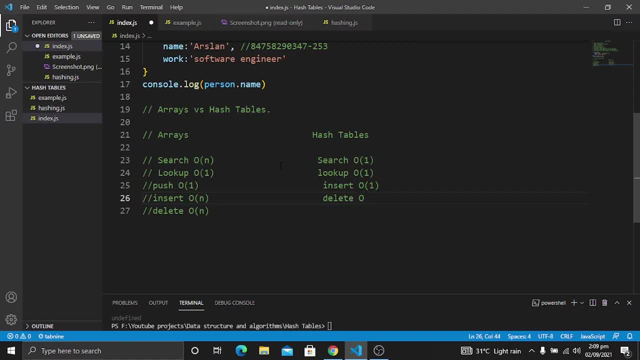 So it will be a deletion will also be of one. So you can clearly, on this basis, on the basis of the time complexity, you can compare the arrays and the hash tables. So the arrays have a linear time complexity for searching, inserting and deletion. 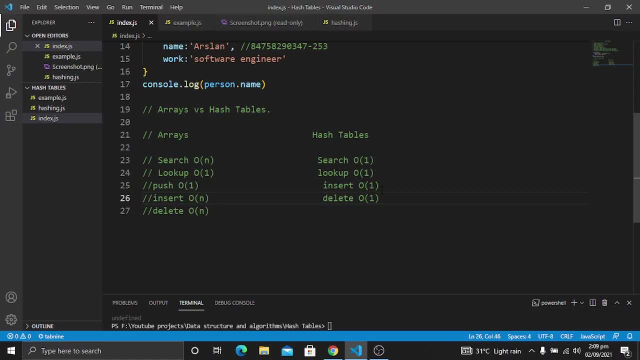 So these are the expensive things in arrays, Whereas in hash tables these are not expensive things. These are fast. That's why we use hash tables in databases And what we can say. the lookup and the pushing or appending the data is not expensive. 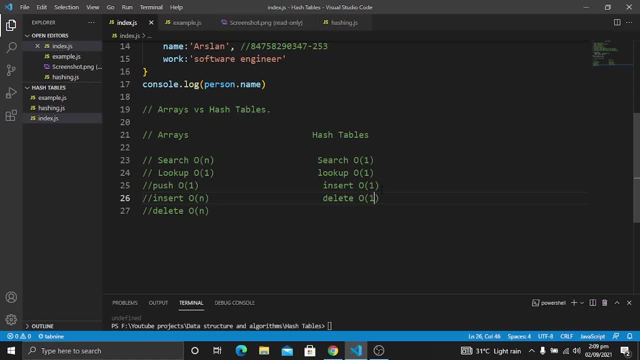 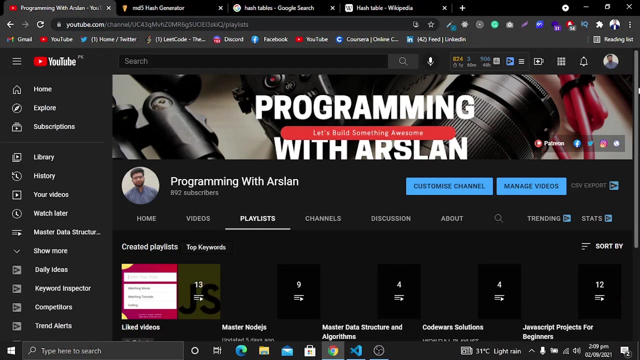 It has the constant time complexity in arrays. So these are the difference between arrays and hash tables. I think you have, I hope you have learned something from this lecture or this tutorial, and this tutorial will be added to This data structures and algorithms playlist. 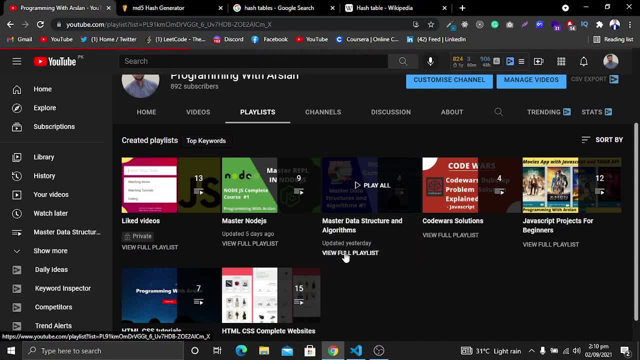 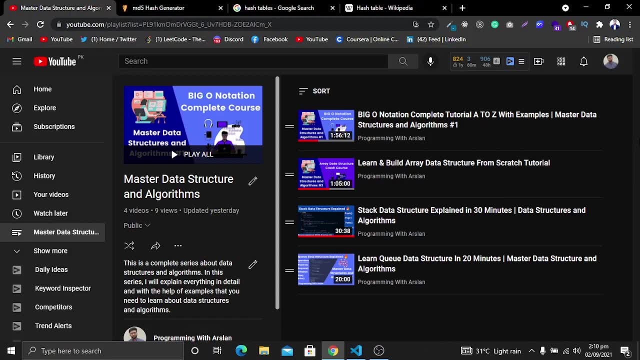 So this playlist is here with the name of master data structures and algorithms. So this is the complete data structures and algorithm score in which we can cover all of the topics- All of the main are the topics which are usually asked in coding interviews- And we will also cover the questions which will be the interview questions in the later part of this series, when we will complete the data structures and algorithms. 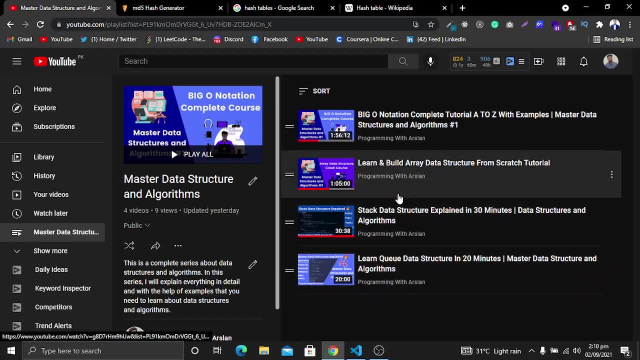 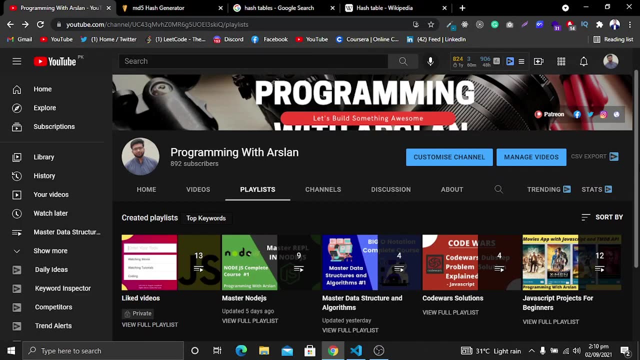 So this tutorial will be added here, and in the next tutorial we will cover some next topics about the DSA. So don't forget to like the video, subscribe to this channel and please comments in this video What kind of knowledge you want or what kind of things that you don't understood, and you want me to make a video on these topics. 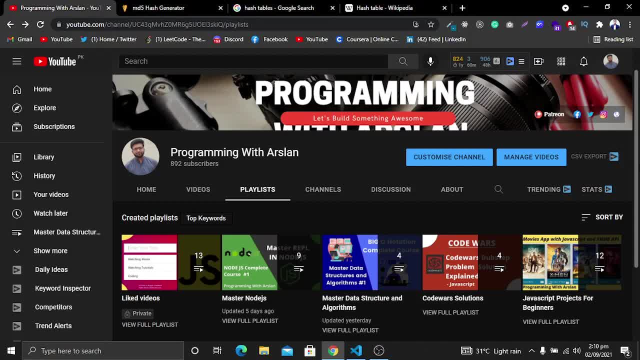 So give me the topics in the comments and I will make a video on your topics. and also tell me in the comments what you have learned from this video. What are these confusions that you have removed after that has been removed from your mind after watching these tutorials? 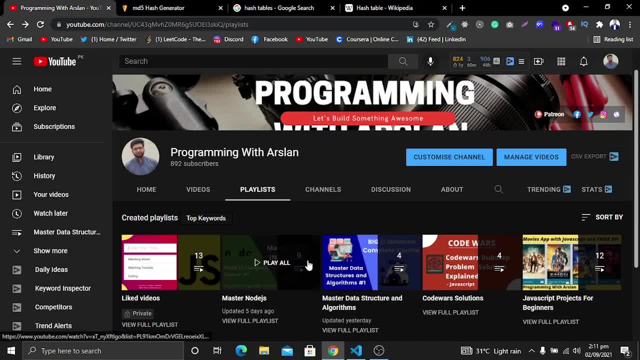 So I hope you have enjoyed this video. You have learned something new from this video, So this is going to be the end of this tutorial. Have a nice day. Have a nice day and bye.